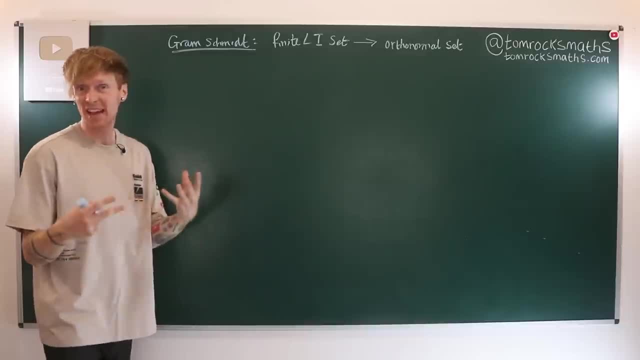 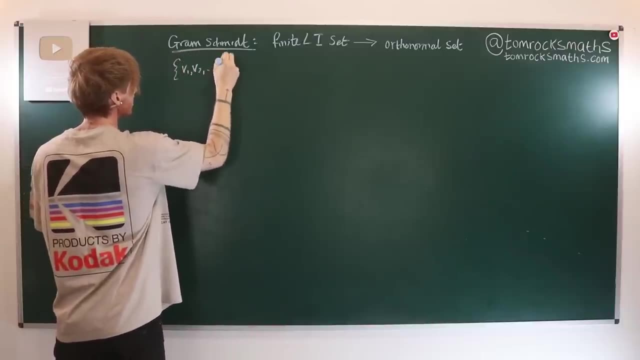 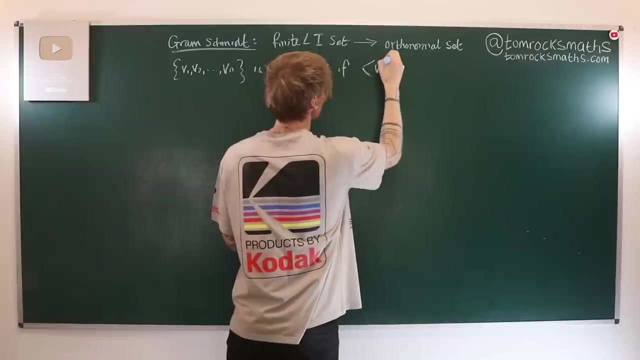 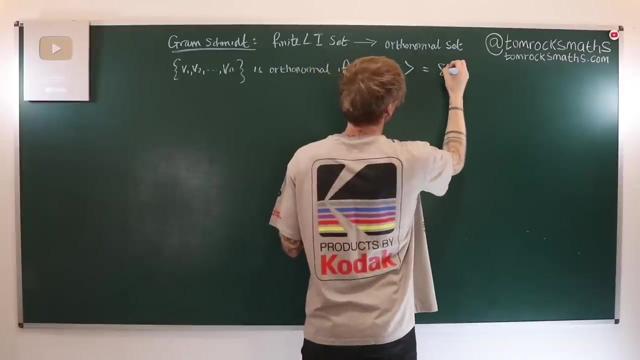 we call the definition of an orthonormal set of vectors as follows. We say that V1 up to Vn is orthonormal if the inner product between Vi and vj, so any two members of the set, is equal to delta ij, where the delta function gives you. 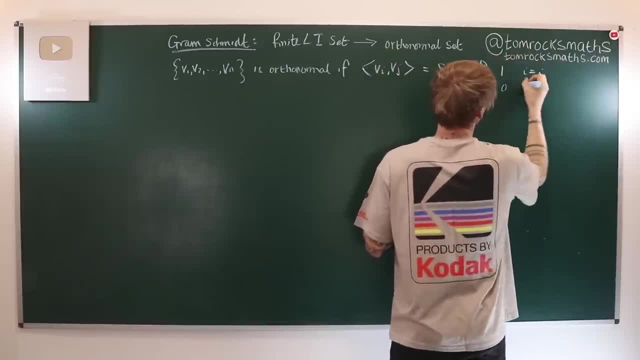 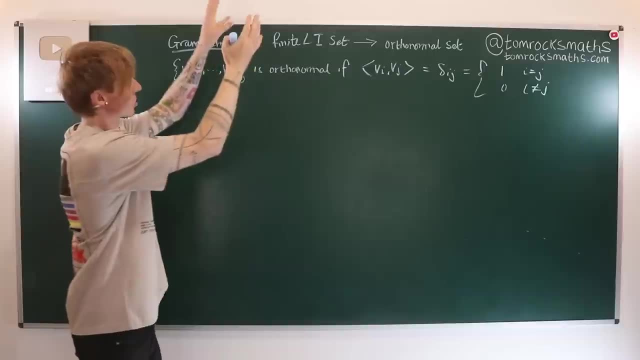 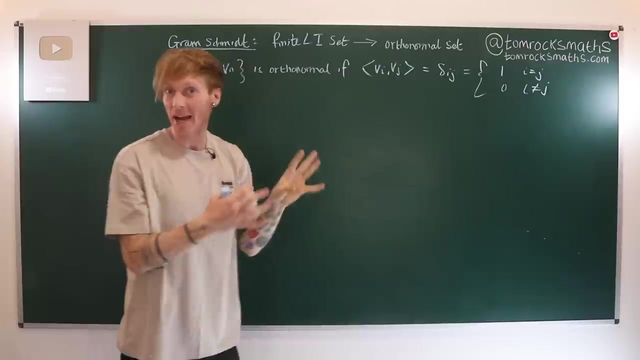 1 if i is equal to j and 0 otherwise, so ie if i is not equal to j. So, Gram-Schmidt, start with our linearly independent set, which must be finite, and then it will output. having followed the steps of the algorithm, it will output an orthonormal set, which means that 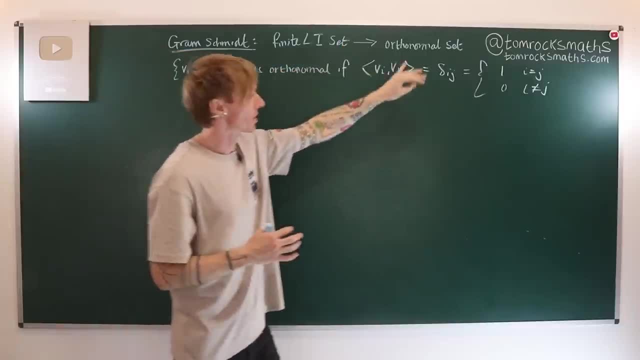 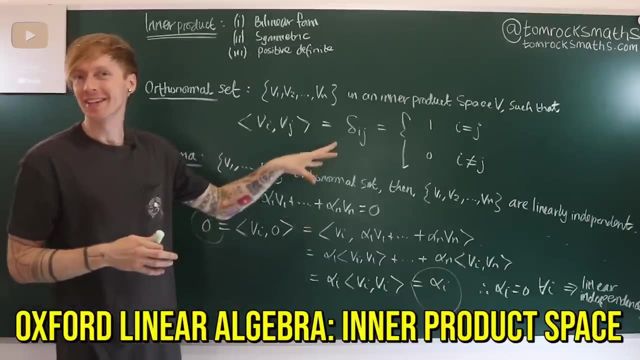 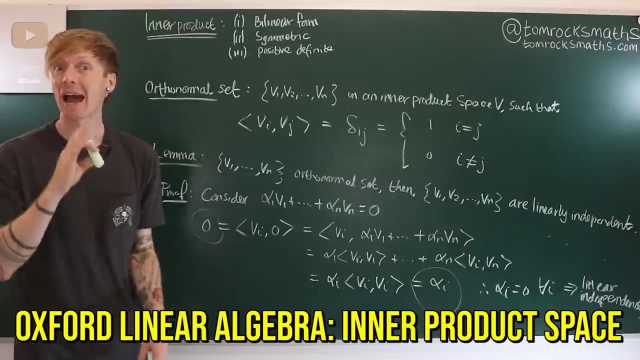 taking the inner product of any elements within this set can only give you 1 or 0 according to this definition. Now in the previous video we actually saw how an orthonormal set within an inner product space is in fact linearly independent. So the Gram-Schmidt process. 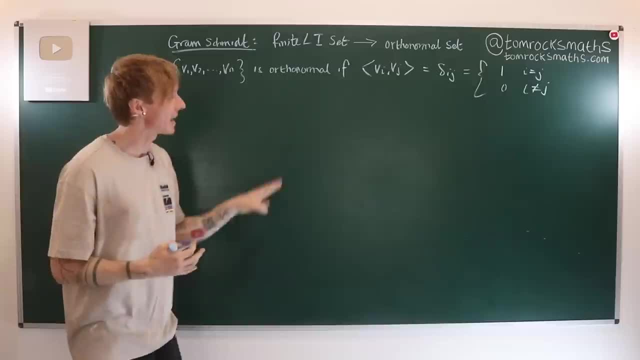 is actually an orthonormal set within an inner product space. So the Gram-Schmidt process is actually an orthonormal set within an inner product space. So the Gram-Schmidt process is actually playing the role here of the converse. It's telling us that if we start with a linearly independent set, we can in fact get the orthonormal. 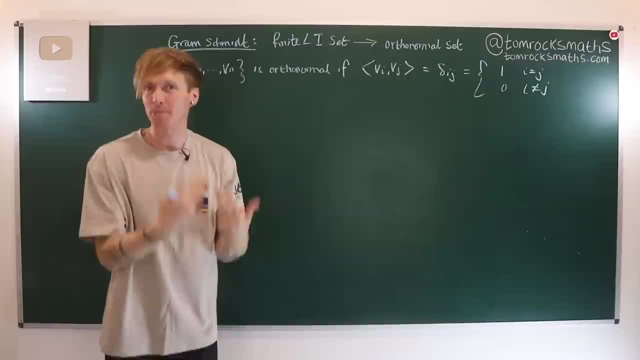 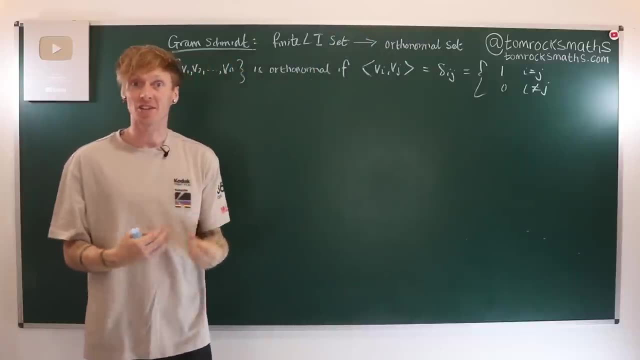 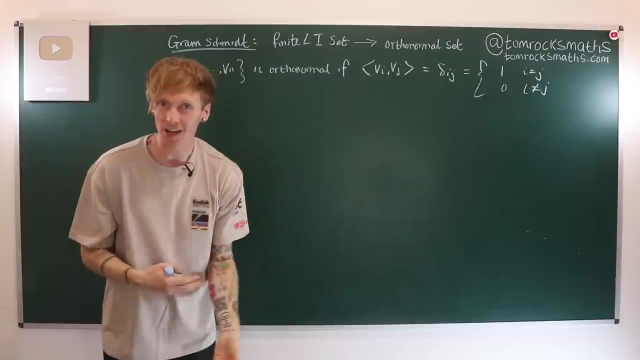 set and, importantly, it actually gives us an explicit way to calculate exactly what that set is. So not only does it tell us that such a set exists, starting linearly independent, we can always get orthonormal- it actually gives us a recipe to follow to calculate those vectors. 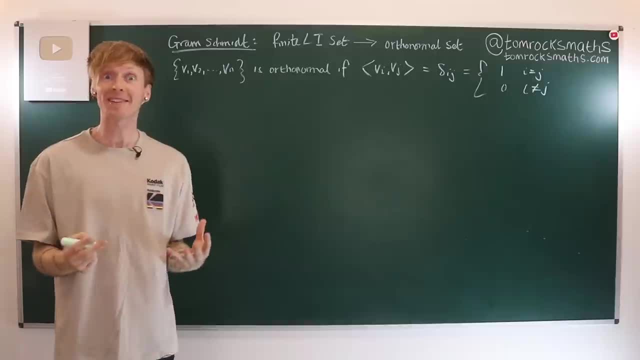 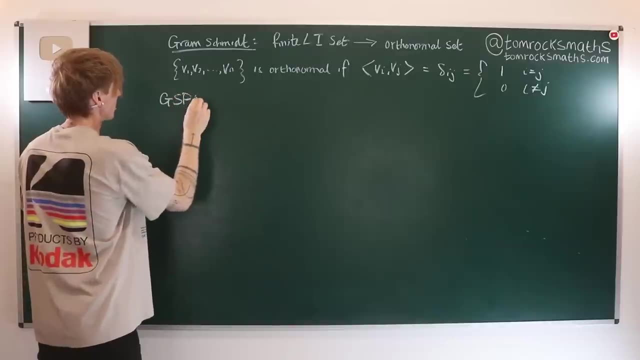 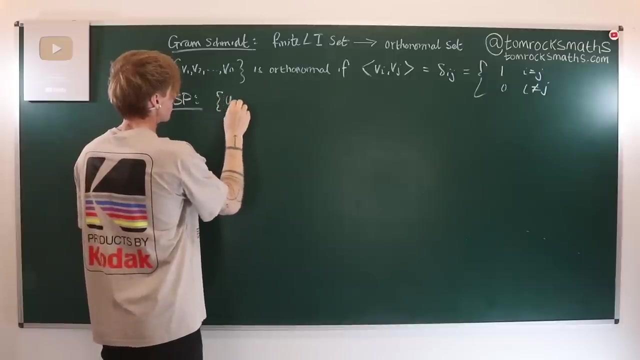 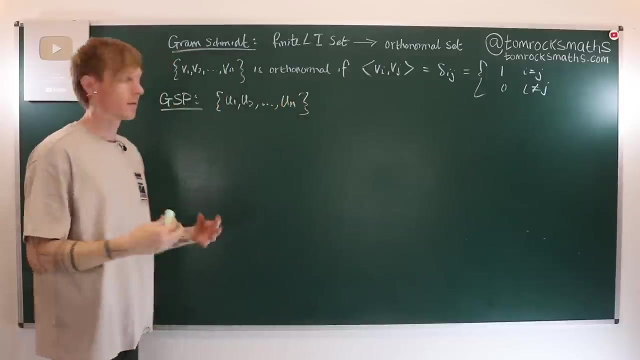 those orthonormal vectors explicitly. So here are the steps of the Gram-Schmidt process, which I'm going to write as shorthand, gsp. So, as I've written at the top, we begin with our linearly independent set- let's call it u1, u2, up to un, and step one is simply to take: 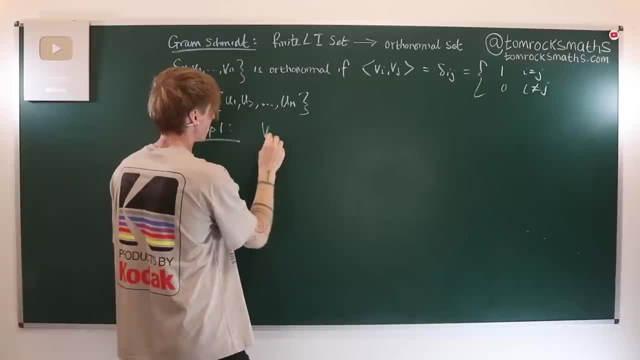 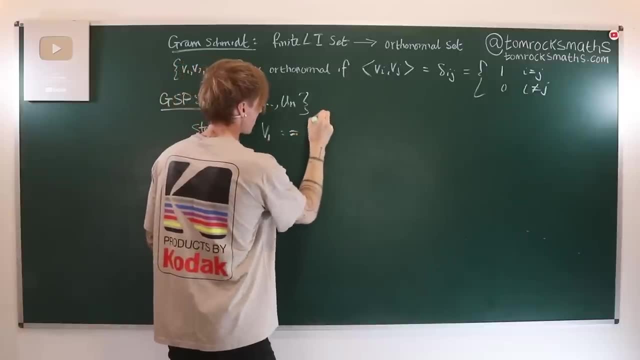 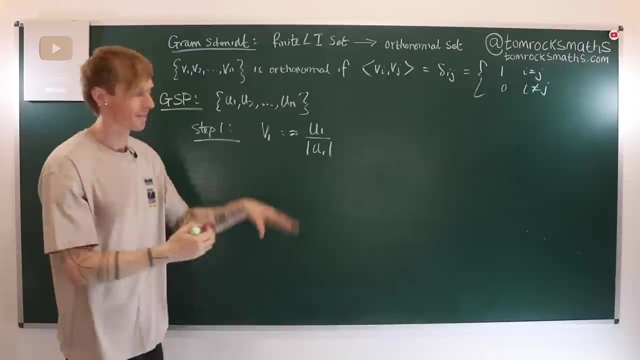 our first vector, u1, and what we need to do is define v1, our first orthonormal vector that is just going to be given by the vector u1 divided by its norm. So here we are normalizing the vector, which means that when we now take the inner product of this thing with itself, we will indeed 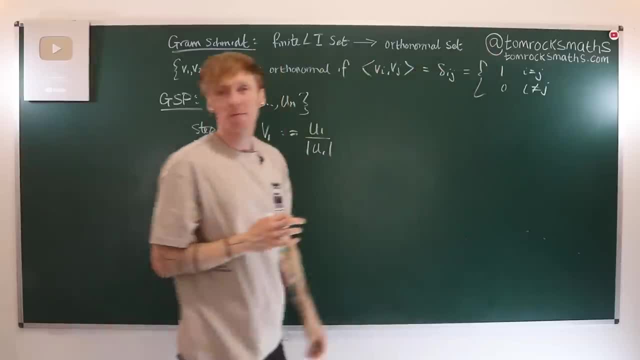 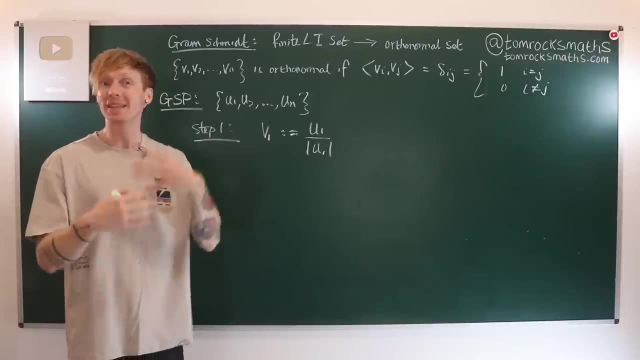 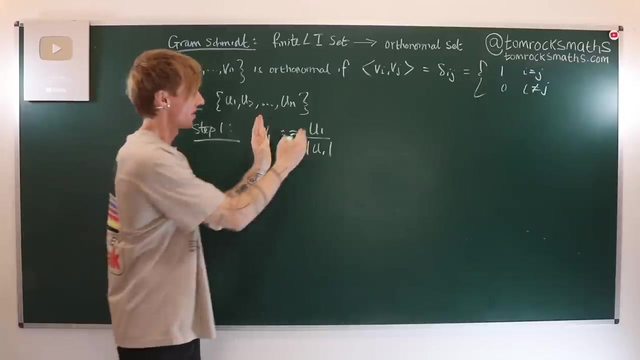 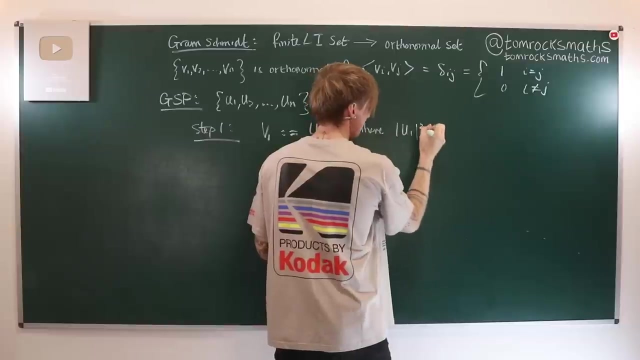 get one. so we're making sure that this property up here is satisfied. Now, anytime we do a division in any kind of calculation, you should be thinking: could the denominator be zero? and we're actually okay here, because the modulus of u1- so where the modulus of u1 squared, we actually say, is the inner product, u1 with itself. 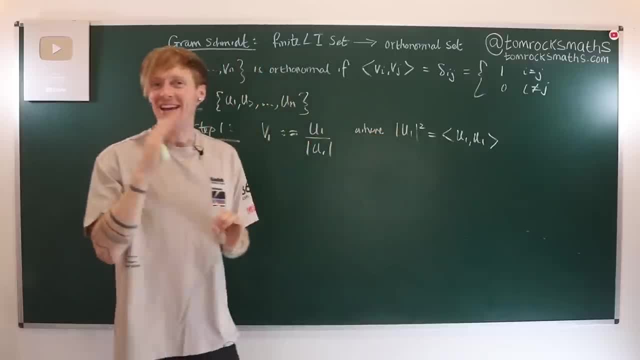 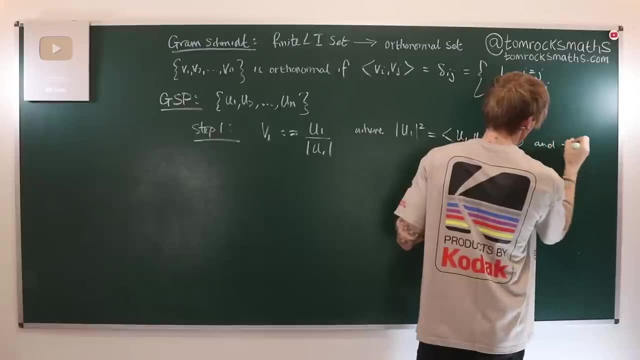 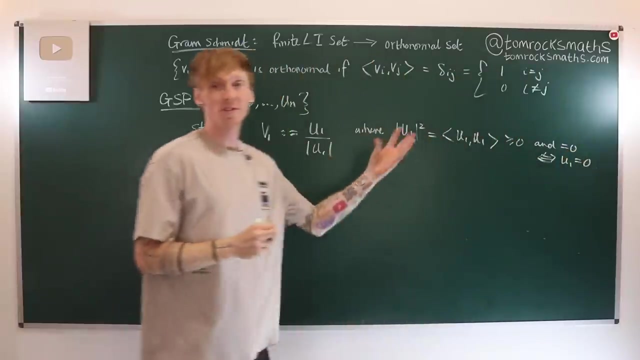 and, of course, by the fact that this is an inner product. we therefore know it is positive definite. so we know that this is greater than or equal to zero and equals zero only when the vector itself is zero and of course, the zero vector would not be included in our linearly. 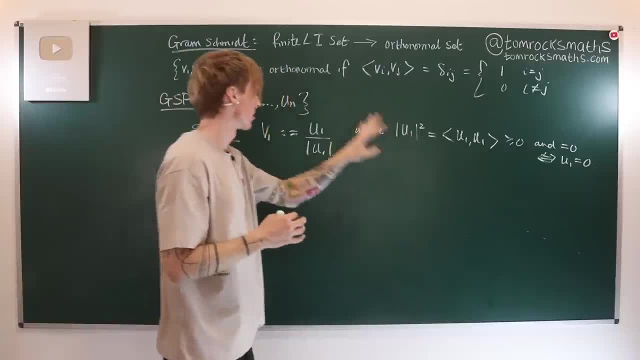 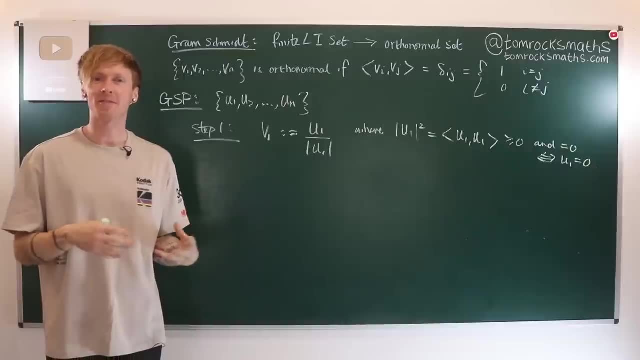 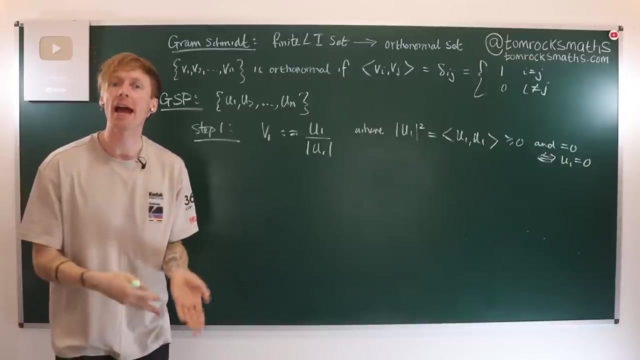 independent set. so by positive definite, we are okay, by dividing by the norm of u1.. Now for step two in the process, and in fact all preceding steps, we are going to form an intermediate which we're going to label with w and then, once we've calculated that, we're going to normalize to get. 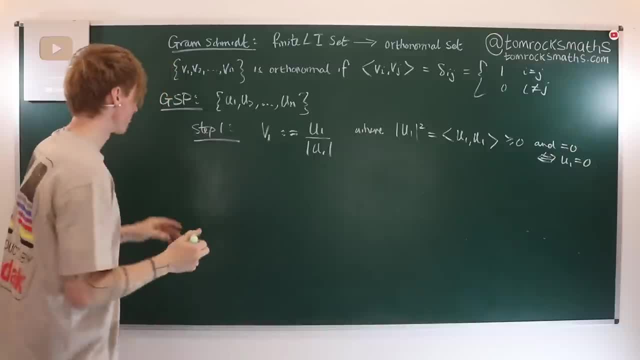 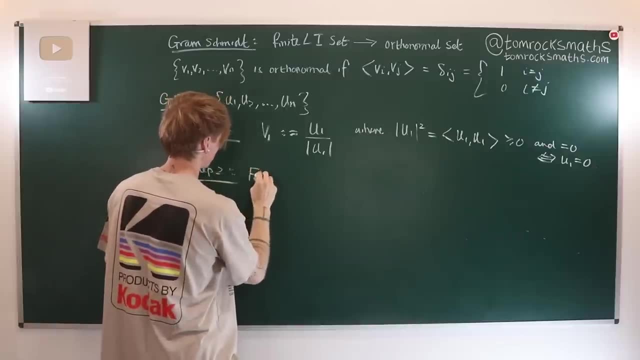 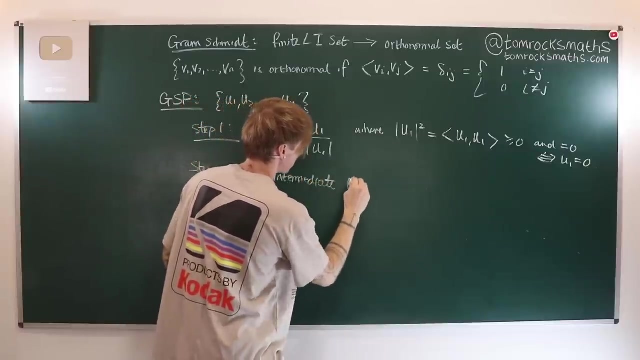 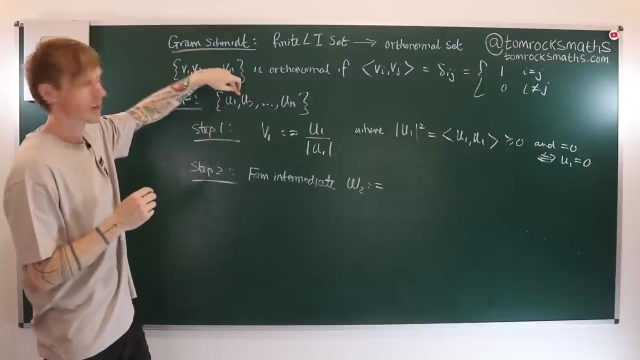 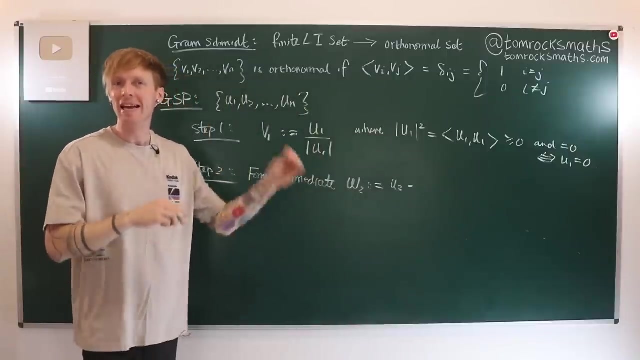 our v, our orthonormal set. So what I mean is as follows: step two is we form the intermediate w2, and the way we do this is we take our second independent vector, u2, and then we subtract off the component of u2 in the direction of v1. 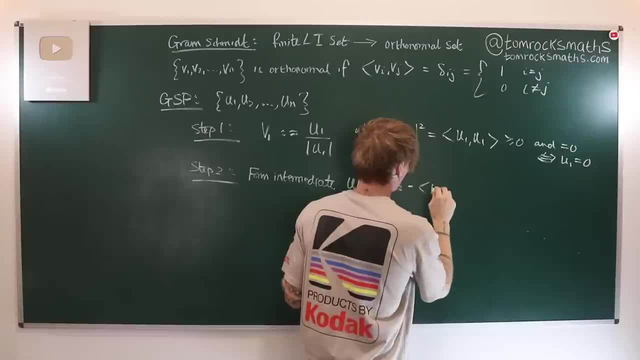 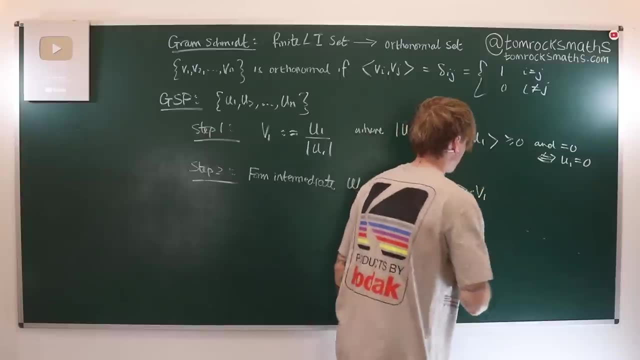 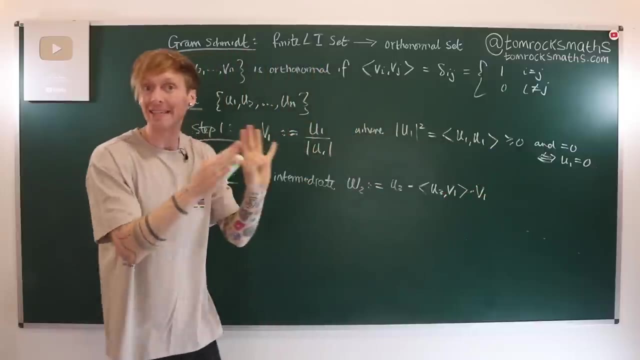 and the way we get that is we subtract off u2, inner product, v1 multiplied by v1, so the inner product gives you a scalar. so we have a vector minus a scalar times a vector. so we're still within v2.. vector space: so everything is okay in terms of our vector space axioms. So this is going to be. 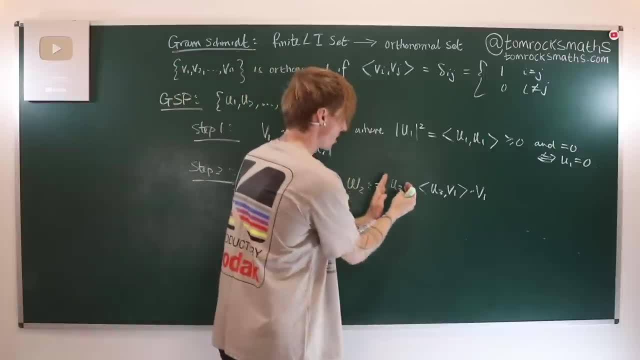 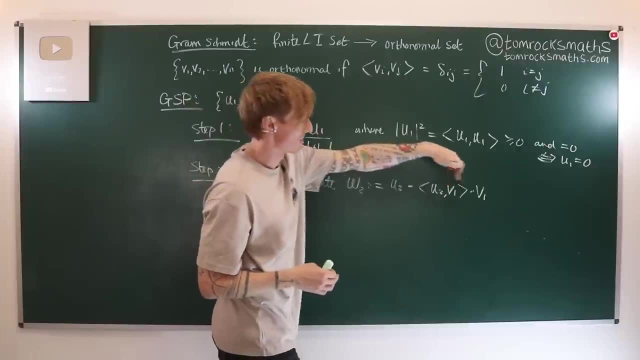 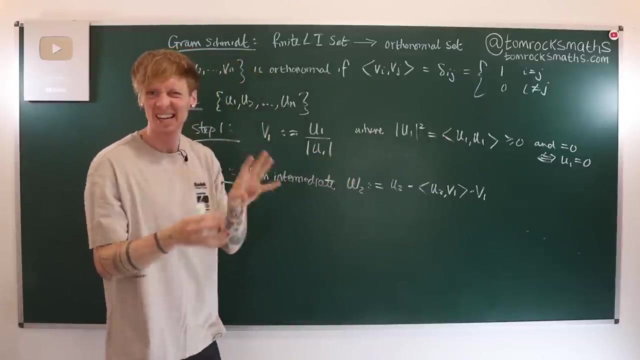 our intermediate. Again, we have taken our vector u2, we've then projected onto the part of it that's in the v1 direction and then we've taken that away. So that's actually going to help with this orthogonality, as we'll see in just a moment when we investigate this a little further. But at 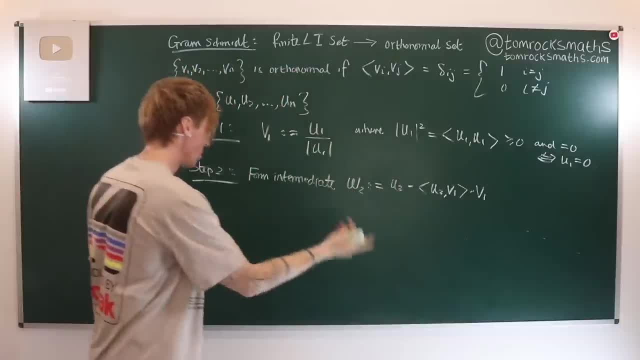 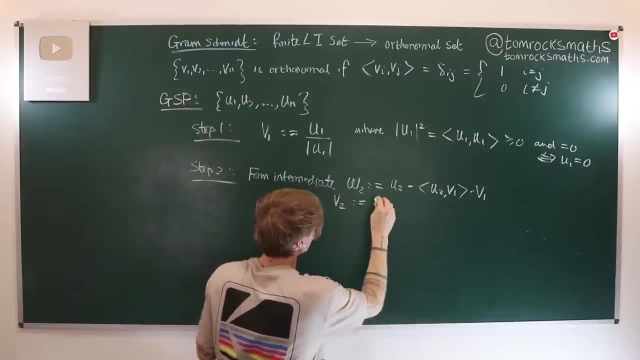 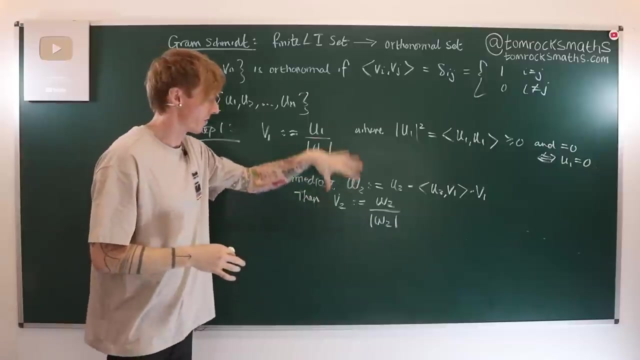 this stage we calculate this and then, once we form the intermediate, we then define v2 to be the intermediate divided by its own norm. Again, to ensure that when we take the inner product of v2 with itself, we're going to get one and satisfy the orthogonality. 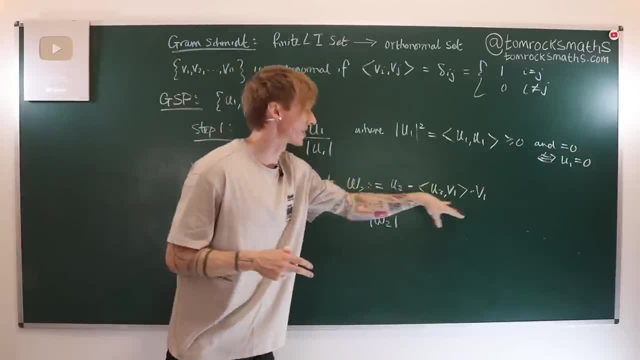 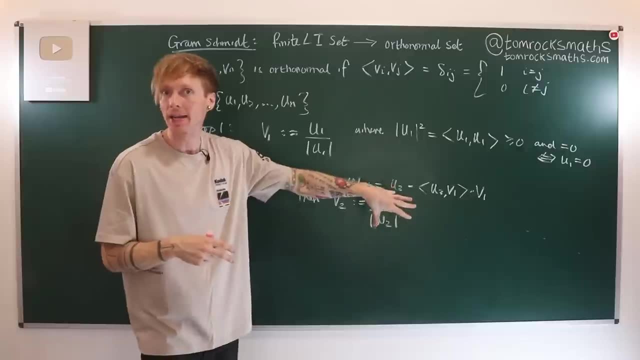 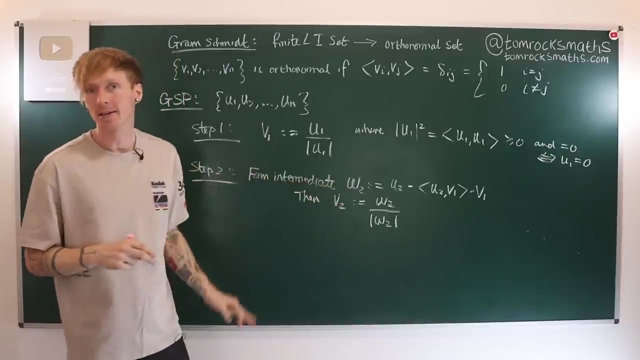 Now let's just take a moment to look at this intermediate vector a little more closely to try to get a feature for what is going on and, in fact, why this is going to work, and give us the orthogonal relationship between w2 and v1.. So what we're doing here is forming 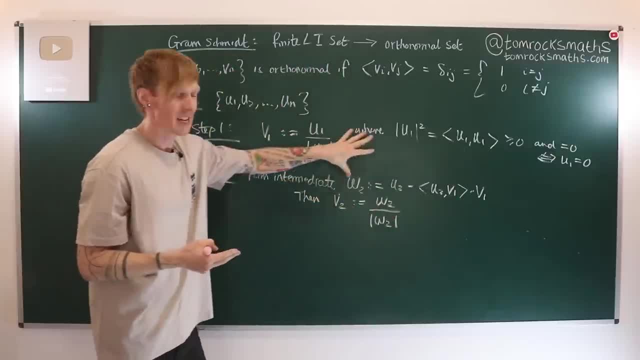 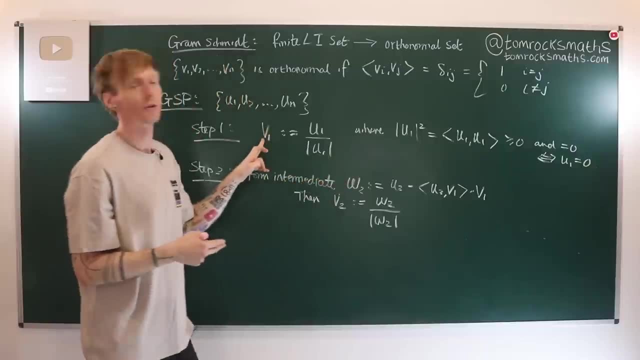 this intermediate and then all we're doing is normalizing it. But even before we normalize, w2, if formed correctly, should in fact be orthogonal to v1.. That still has to be true. Their dot product is going to be zero. that will be true. 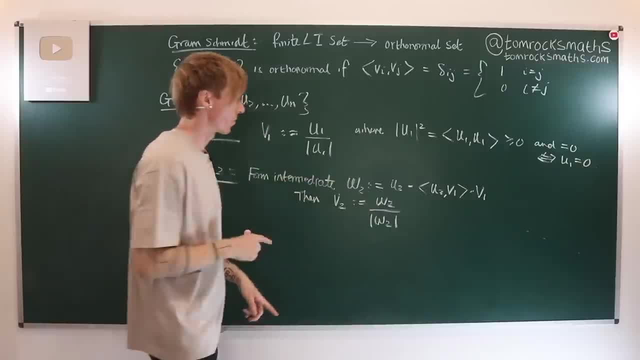 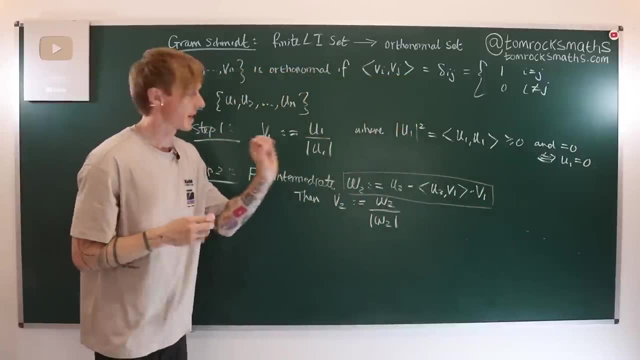 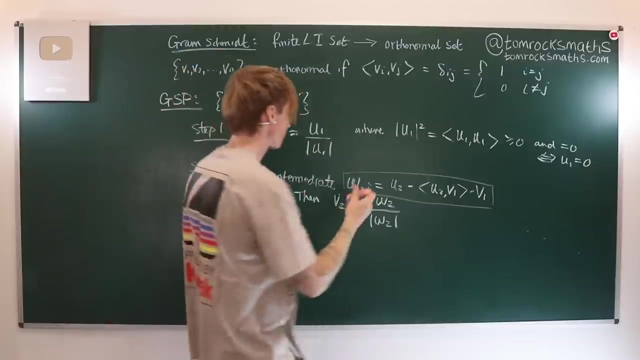 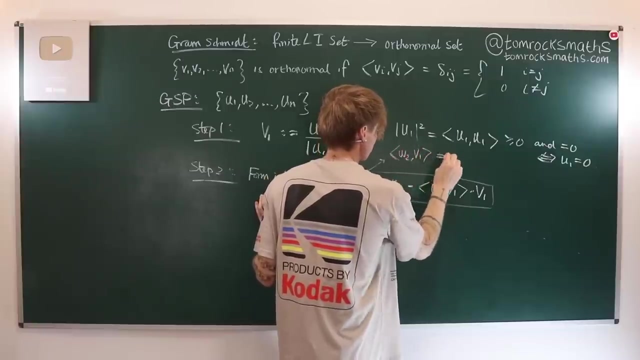 whether or not we divide by the norm. So if we actually take w2 and now calculate explicitly its inner product with v1, we should get zero if what we've done is going to be correct. So we can check that. So let's calculate w2 comma v1.. So we can. 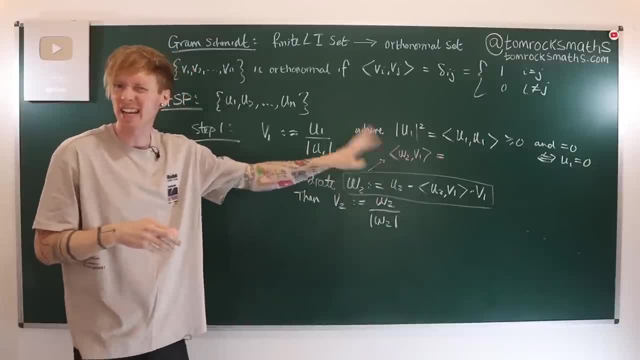 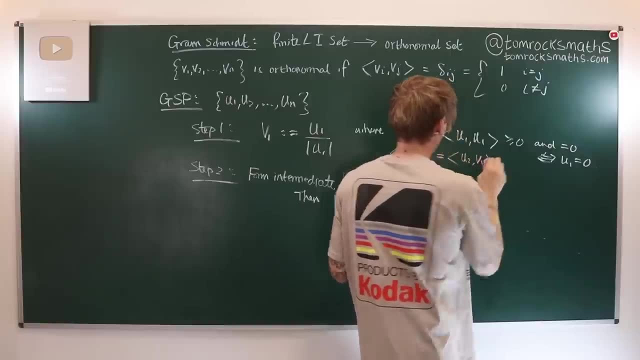 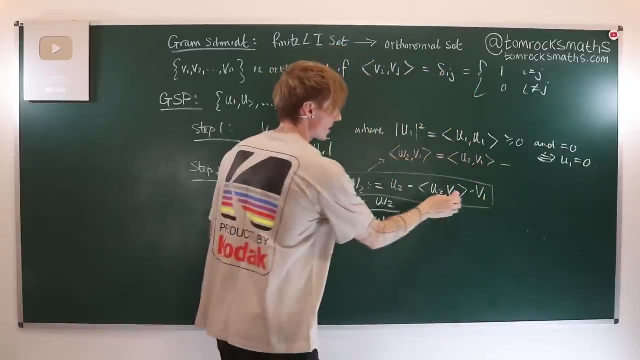 just substitute in the definition and what I'm going to do is just use the linearity as I do. so Just to help a little bit. So we're going to get u2 with v1 from that first component and then what we want is minus. This thing here, remember, is a scalar, so 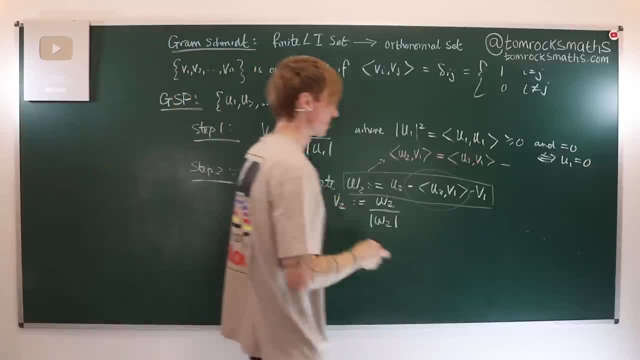 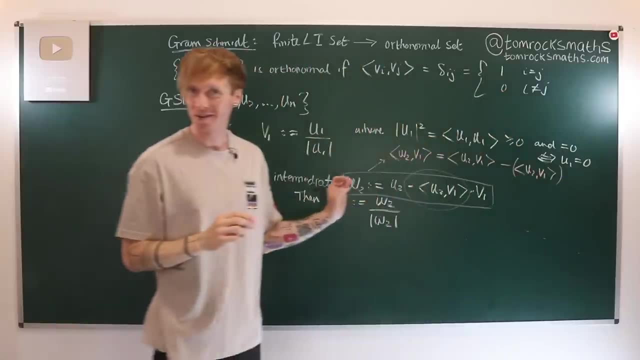 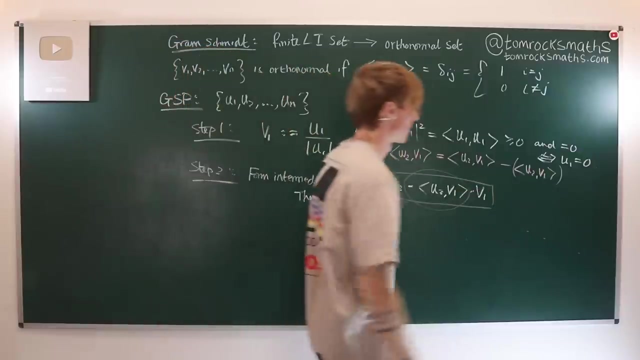 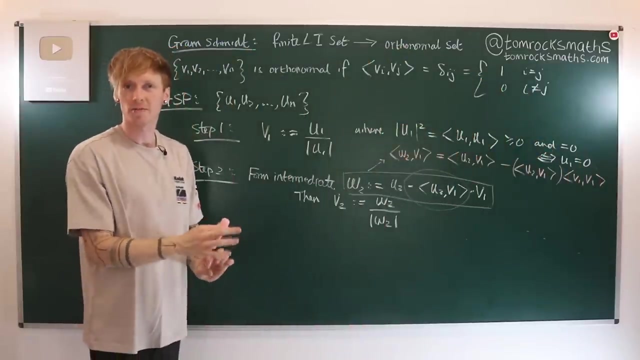 it comes outside of the inner product. So it's minus u2, v1, which is outside of the inner product, And then the inner product we're left with is the vector component v1, which is now with itself, with v1.. So again, just to sort of go over that All, 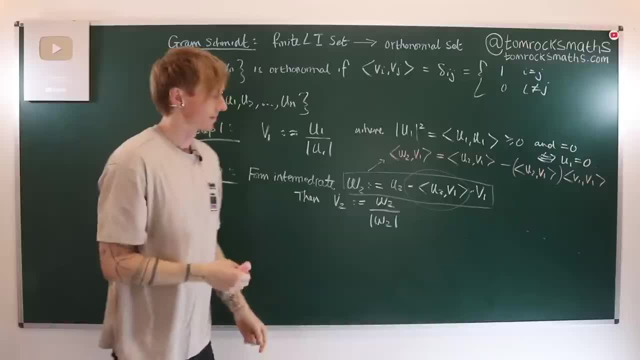 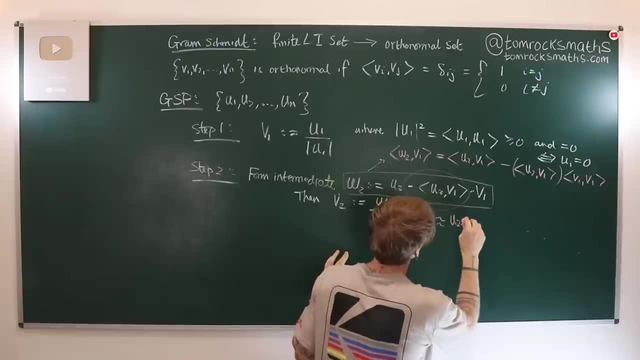 I've done is substitute for w2 into the inner product. Now there are two pieces here and you can sort of, if it helps, think of it as this is basically u2 minus some alpha times, v1.. It's just two vectors where we're subtracting alpha of the 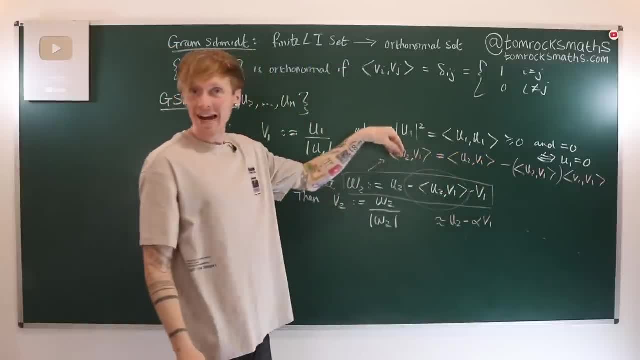 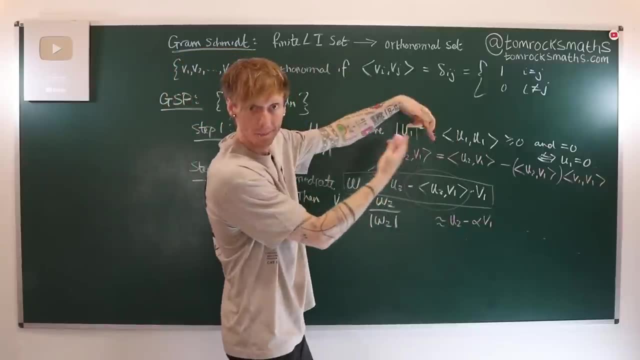 second one from the first one. So now, using linearity, which is one of the properties of our inner product, I can split this up into the first piece with v1 and then I subtract off. this thing here is playing the role of alpha, and 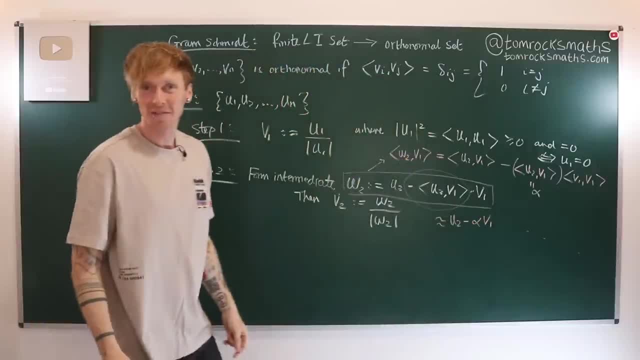 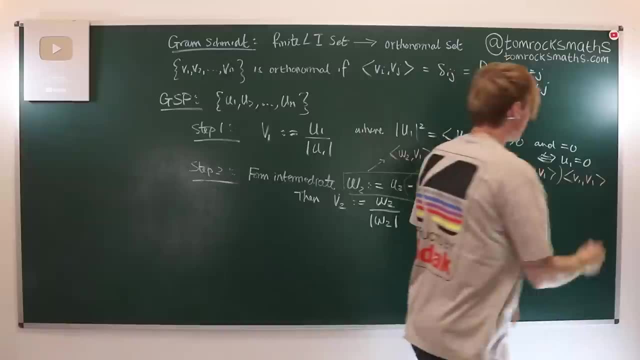 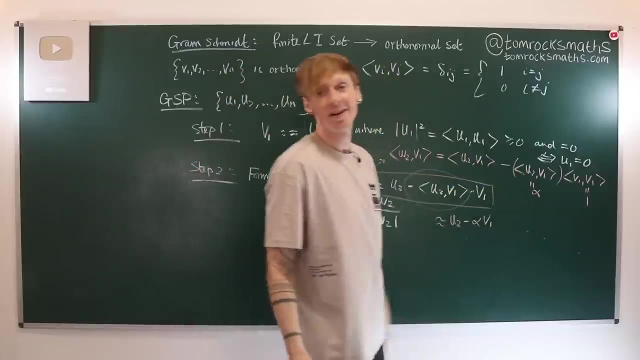 then I'm left with v1, inner product with itself. But of course we have already normalized v1 up here, so this is just 1.. So what we're left with is u2 comma v1 minus u2 comma v1.. So we are going to indeed get 0, put a tick there. 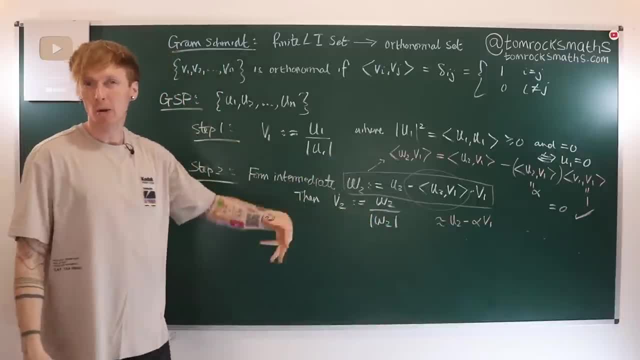 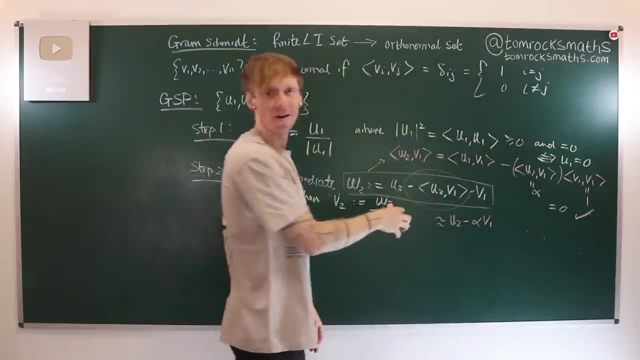 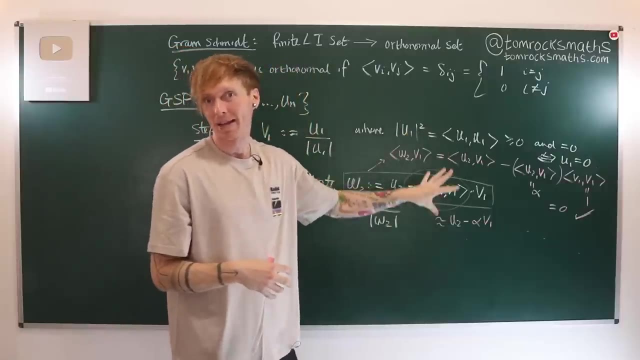 the orthogonality relationship there is going to hold. And it worked precisely because we subtracted off alpha lots of v1, where that amount, that alpha, had to be u2- v1 to make everything balance. Step 3 of the Gram-Schmidt procedure. 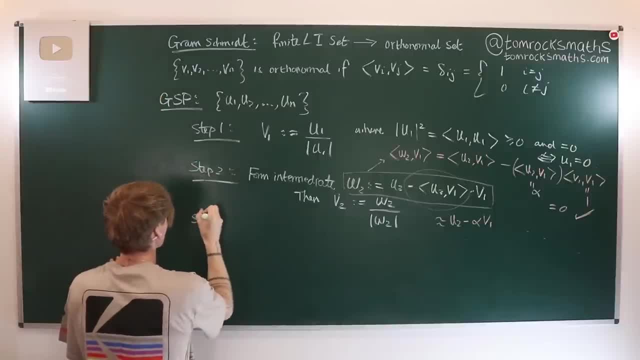 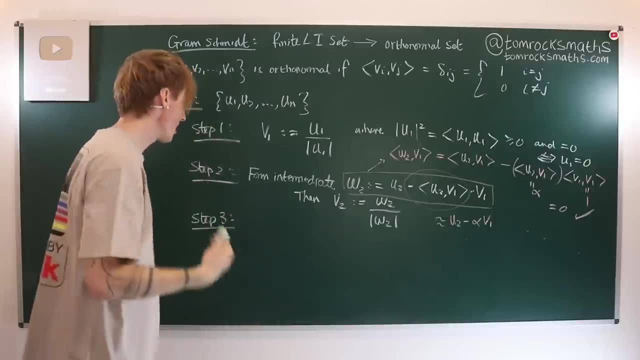 actually just tells us that we've got to make everything balance. Step 3 of the Gram-Schmidt procedure actually just tells us that we've got to basically repeat step 2, but for the next vector in our list. So here, so we. 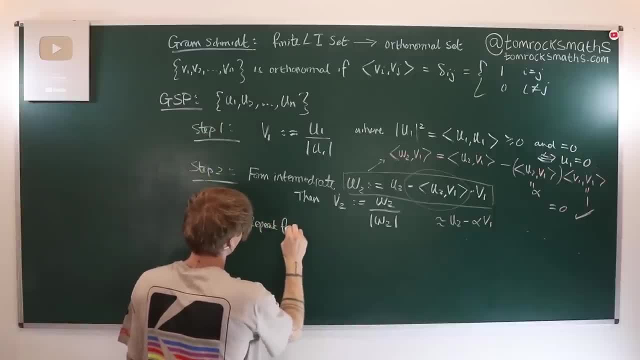 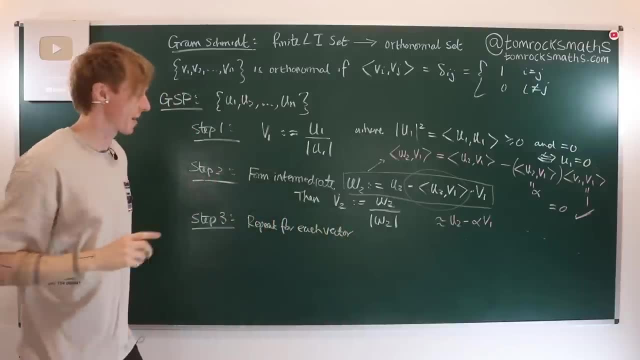 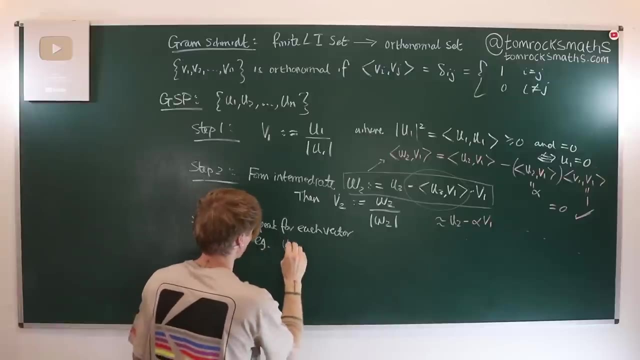 sort of say: repeat for each vector. And what we mean by that is, there is a very slight sort of modification you have to make at each step. So we repeat for each vector. so, eg, for the next one we form the intermediate. So we would form w3 and 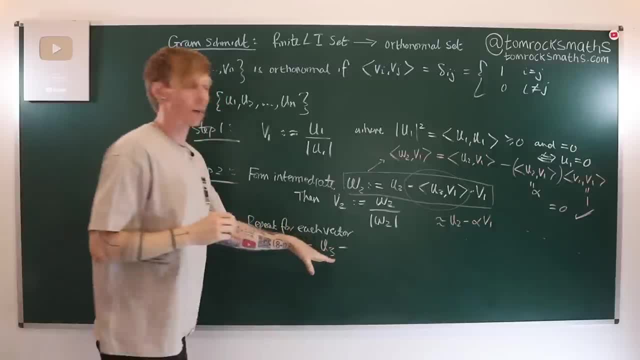 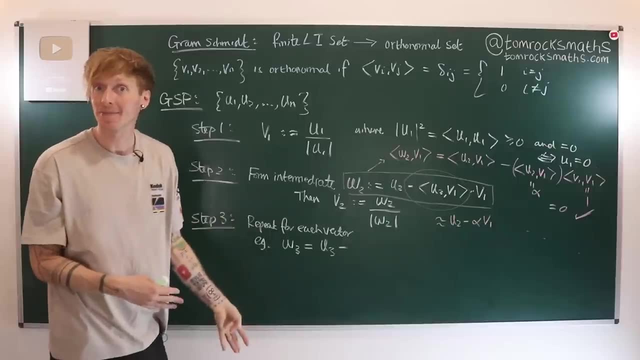 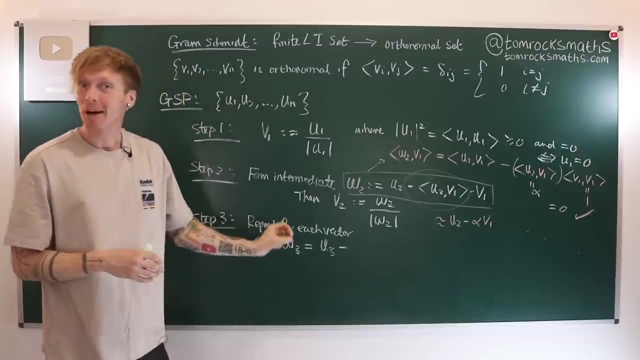 w3 is equal to our third vector. Now we subtract off the components of u3 in the directions of the vectors we've already defined. So we want to subtract off any part of u3 that's in the v1 direction and any part of u3 that's in this v2. 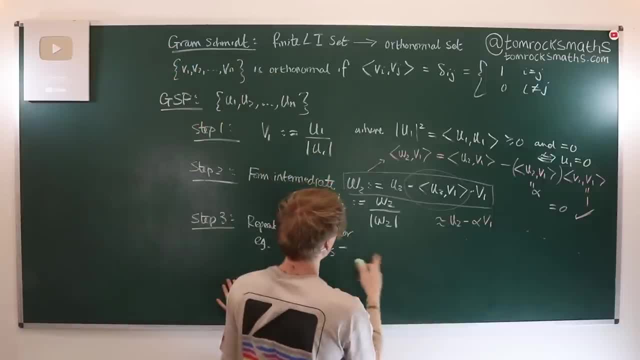 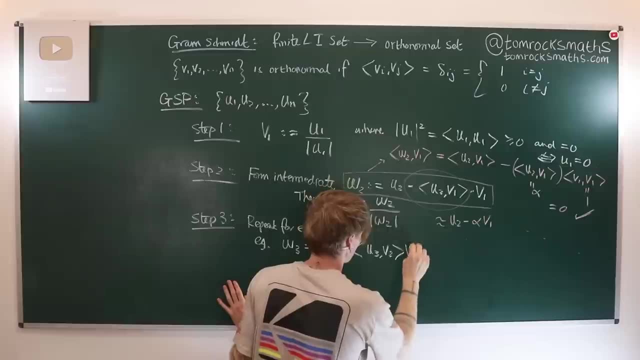 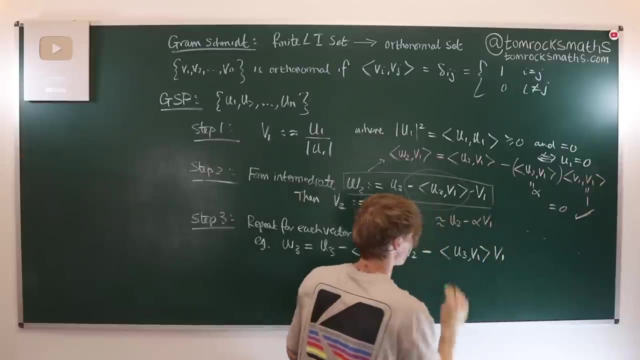 direction. So we want to do u3 minus. let's subtract off the bit in the v2 direction, So that's u3- v2.. And then let's subtract off any part of u3 that's in the v1 direction, where. 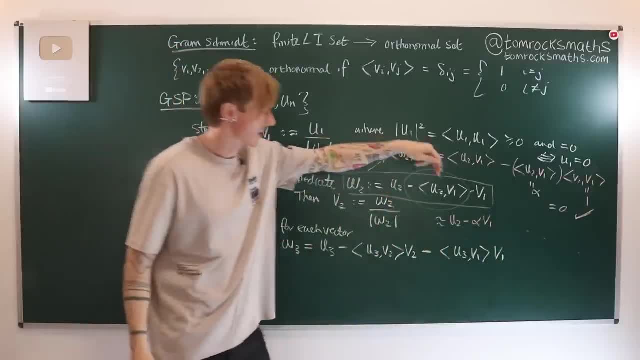 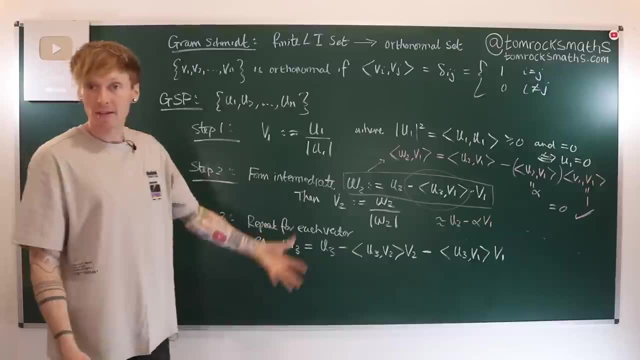 again, the amount of v2 that we subtract and the amount of v1 that we subtract is this projection in a product in both cases. So this is going to be our intermediate, and after we've done the intermediate, we then say: and once we've 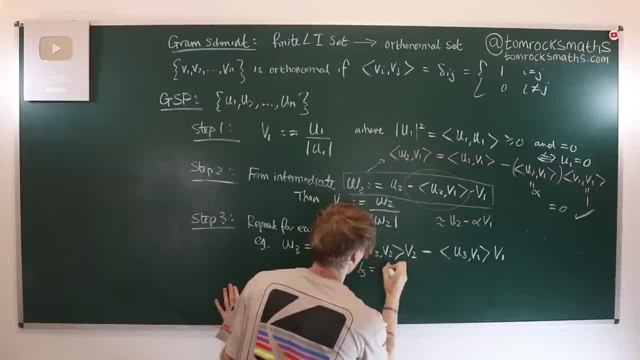 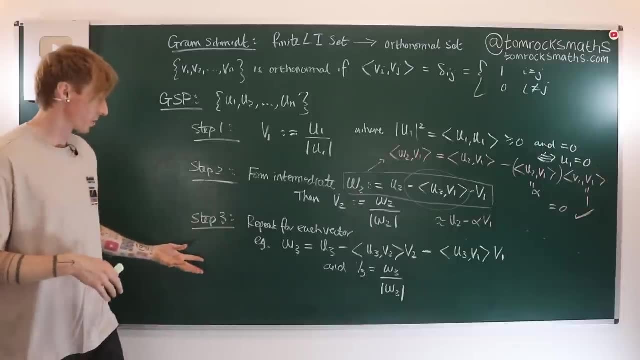 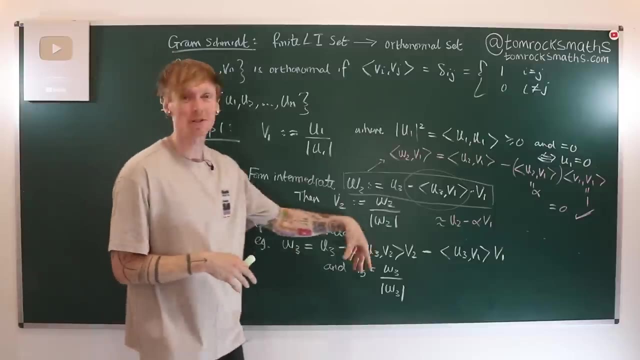 done that, v3 is then just going to be w3, divided by the modulus of w3.. We continue in this way, so next we would go to w4, which would mean subtracting off three previous parts in the directions of v1, v2 and v3, with 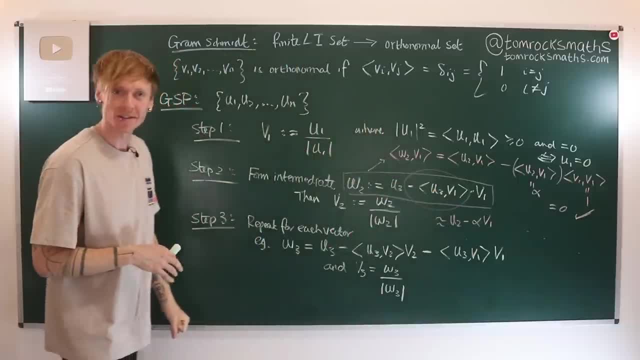 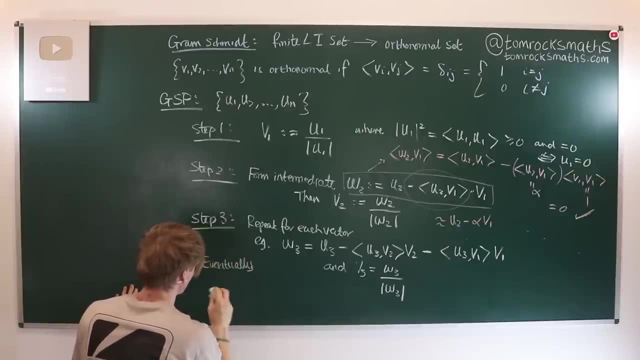 again the same scalar in front of each of those And eventually we would get to the end. So we would eventually get to defining wn, our intermediate, and this would be un minus. now there's going to be a sum of n minus 1 pieces, and each of 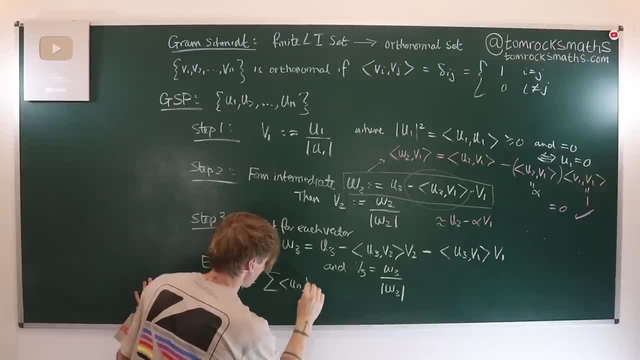 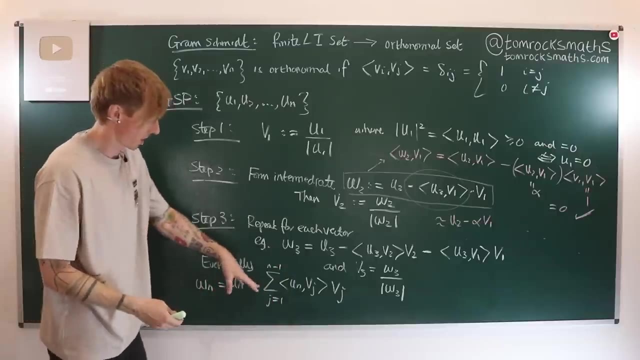 those pieces has a coefficient which is un multiplied by vj, multiplied by vj outside the inner product, And that's going to be from j equals 1 up to n minus 1.. So again, we're just going to subtract off the part of un in the v1. 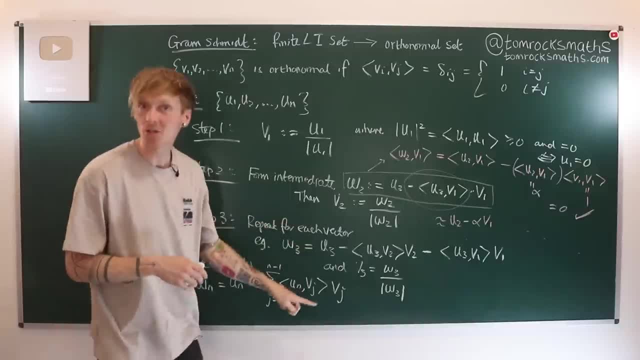 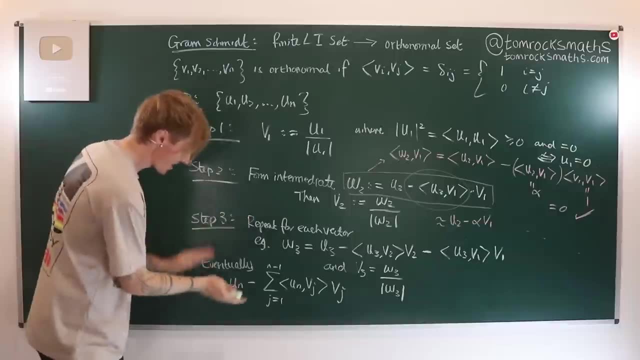 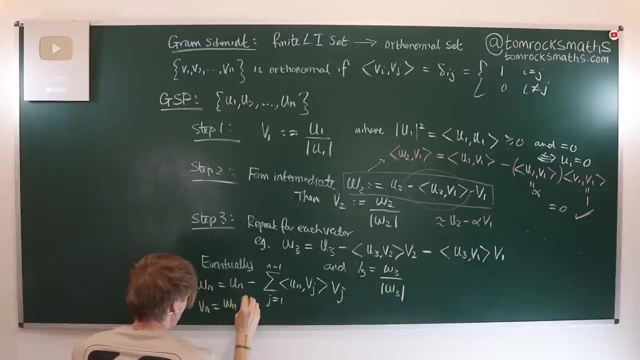 direction, Subtract off the part of un in the v2 direction all the way up to the part of un in the vn minus 1 direction, and then this is wn, and finally we say that vn, our last vector, is wn, divided by its modulus. And that completes the 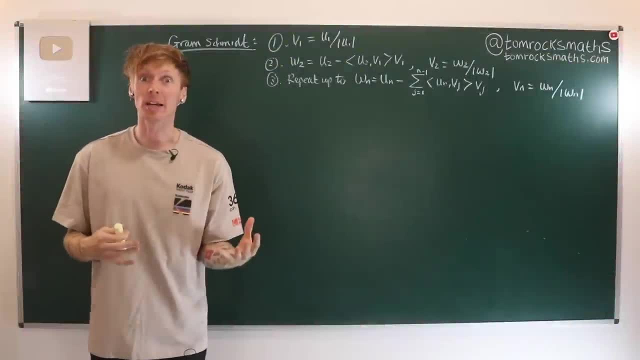 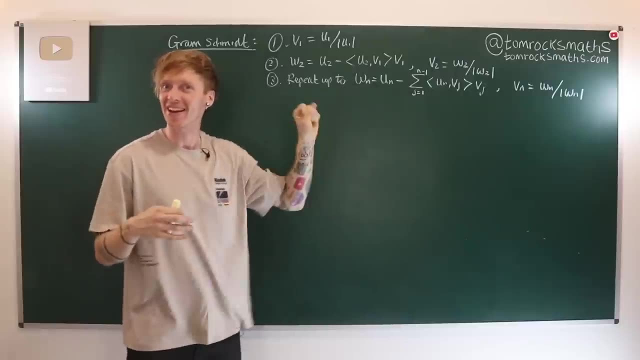 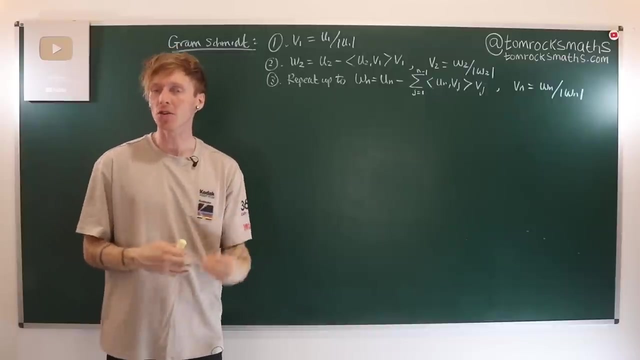 Gram-Schmidt procedure. Now, I did mention earlier that we would look at this concept of projection and subtraction of the previous vectors to get us orthogonality. We're going to look at this in a little more detail with an explicit, concrete example, looking at the. 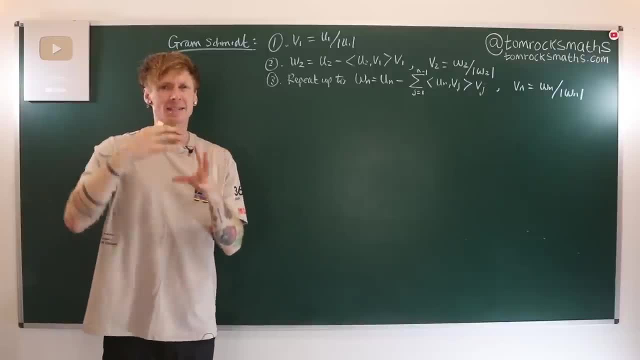 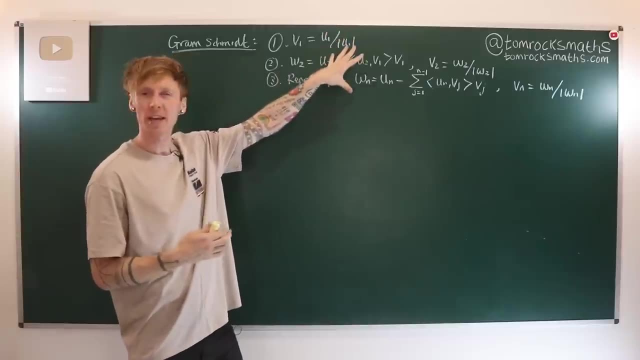 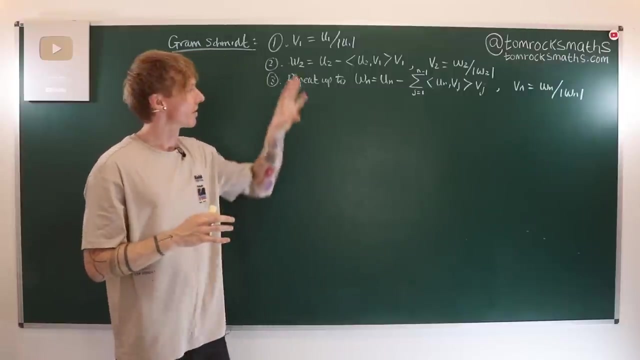 2D Cartesian plane As I know- for me at least, it is very helpful to visualize exactly what's happening here And hopefully, if I can convince you how this works in 2D with our usual Cartesian plane xy-plane, If I can show you why I 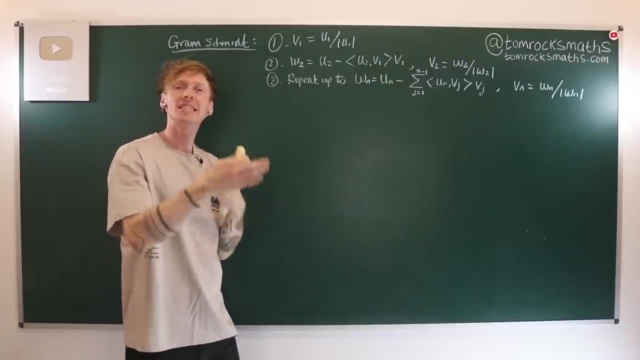 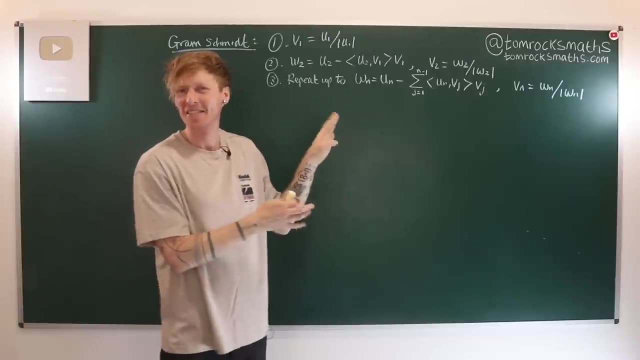 that works and how that works, you can then sort of see how that might generalize into higher dimensions. Unfortunately, I cannot draw 3D and higher very well on this board, which is why we're going to focus on the 2D case. but 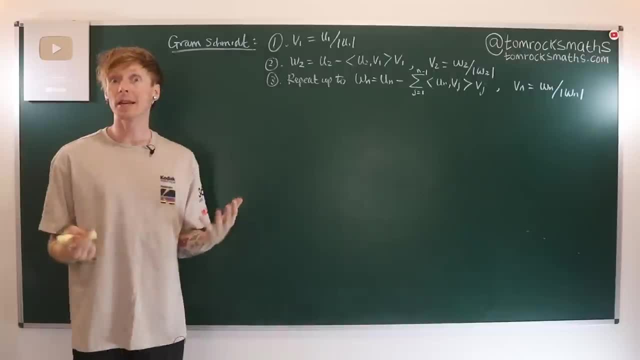 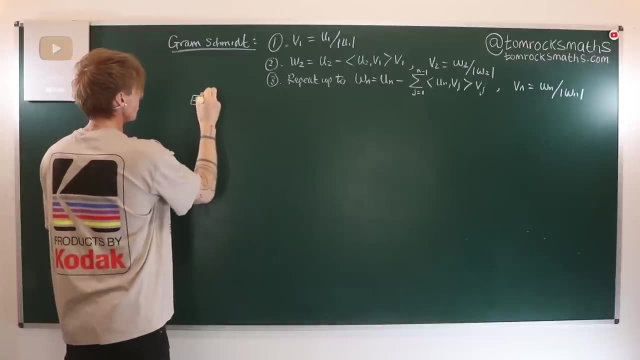 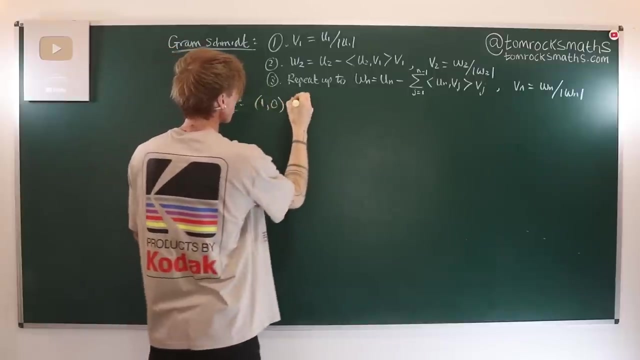 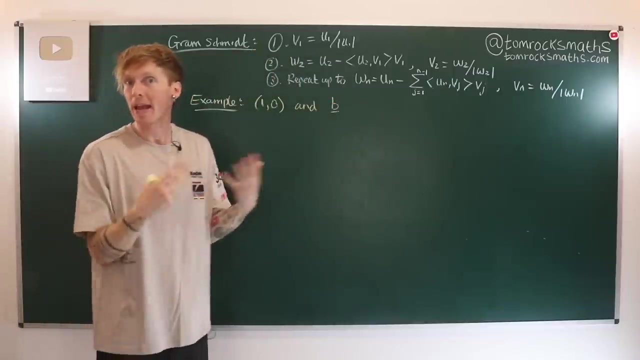 it will generalize in exactly the same way. So let's suppose I have two linearly independent vectors in the 2D plane and they are going to be given by one zero and some other vector. let's call it b, and as of yet b could be anything as long. 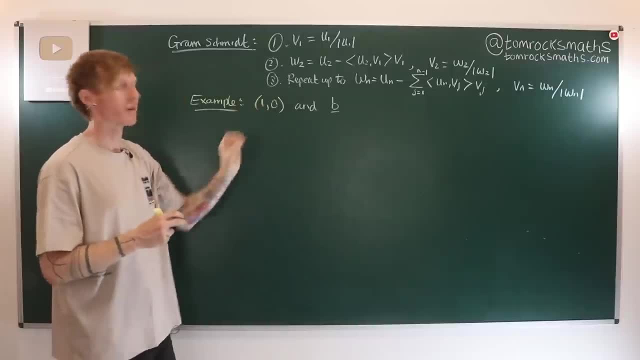 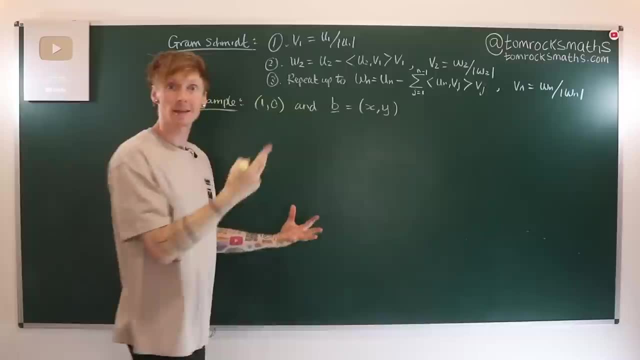 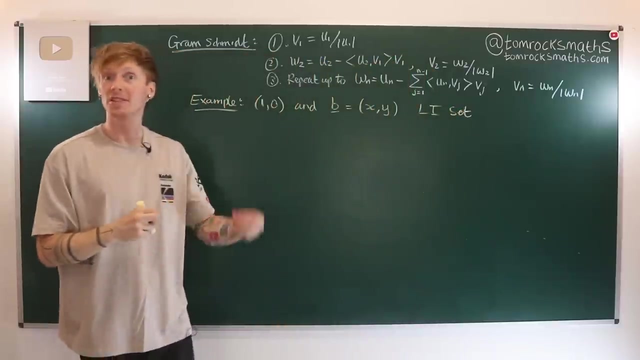 as it's linearly independent with our vector one zero. So let's suppose we're going to call b x comma y. It's a point in the plane, but we know that this is a linearly independent set of vectors because of course that is what we need. 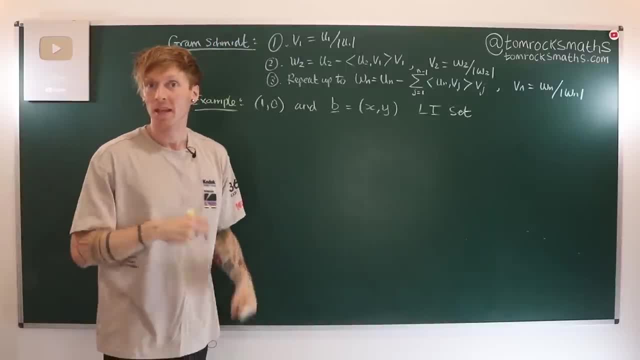 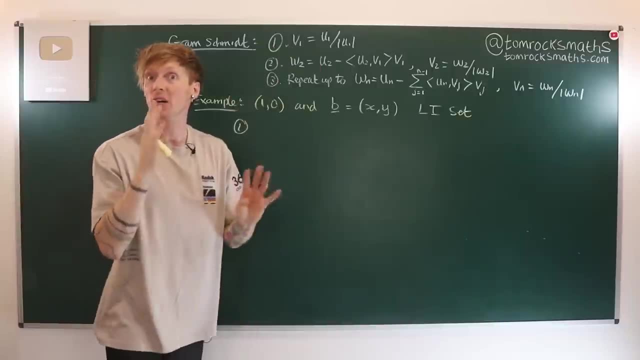 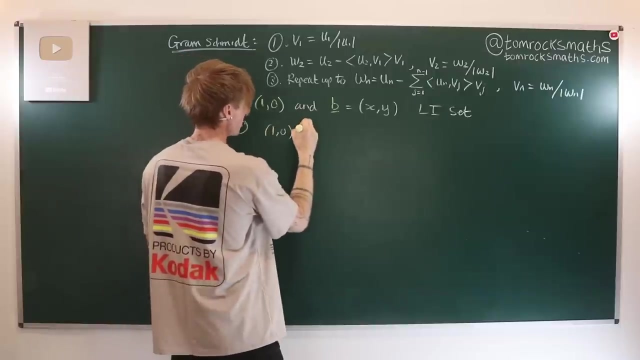 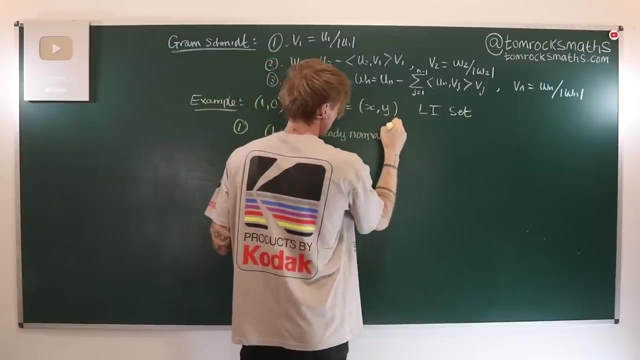 to be able to apply this vector. So according to our steps, Step one: this tells us how to define our first orthonormal vector. but this is already done. So one zero is already normalized. so that's fine, Already has length one. Now step two is going to tell. 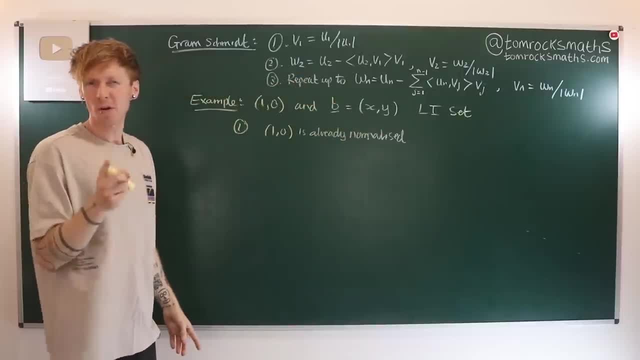 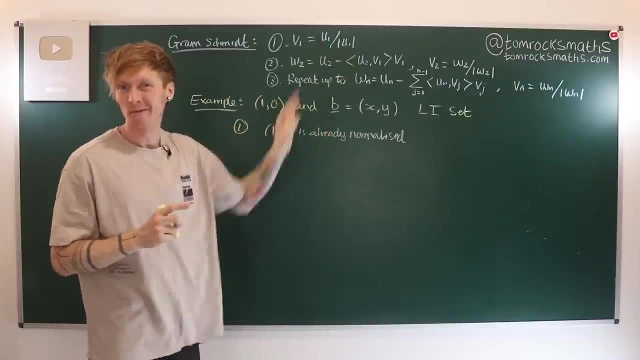 us to compute this particular product. Now, before I do that, I'm just going to draw a diagram of what's happening here, because it's gonna be really helpful again to understand what we're doing. in step two, We have a horizontal vector which is one zero. That's going to be. 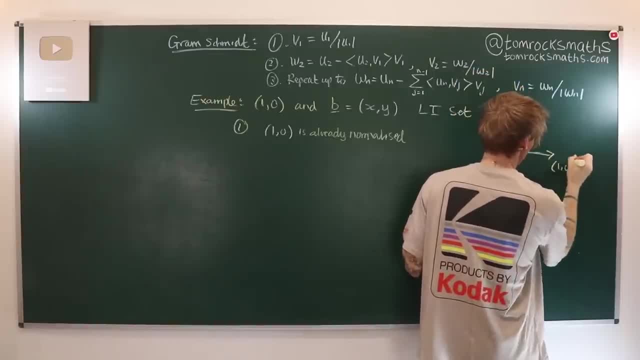 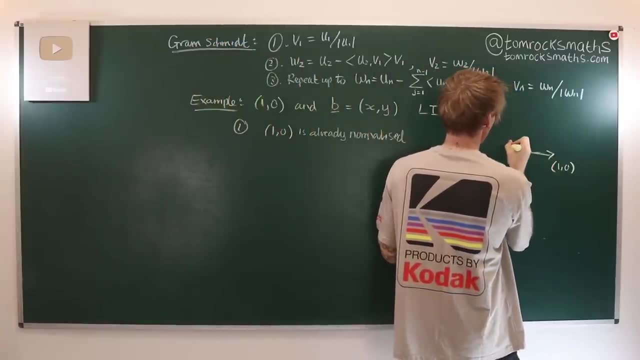 along our x-axis. Let's label that the vector one, zero, And then we have another vector, b, So it's going to some general point: x, y- Let's put this vector up here, like so, And this is going to be the horizontal vector. So we're going to put in the vector y. Let's put this vector up here, like so, And this is going to. 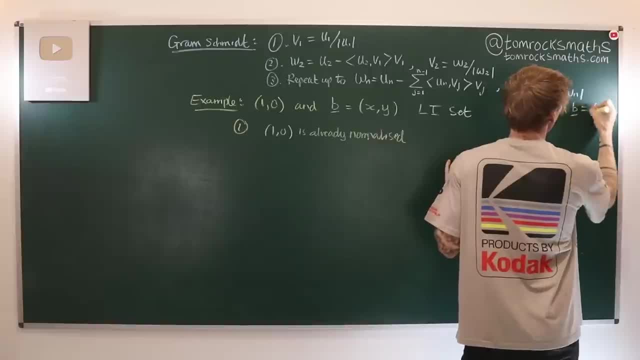 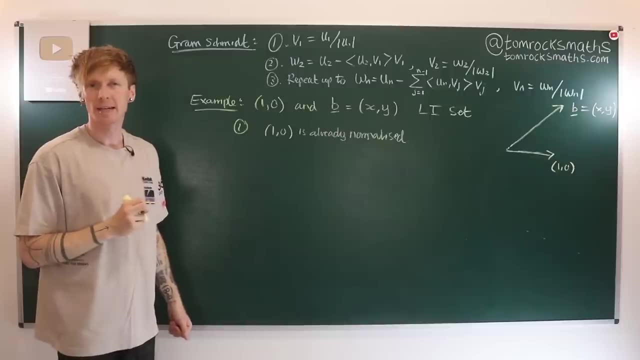 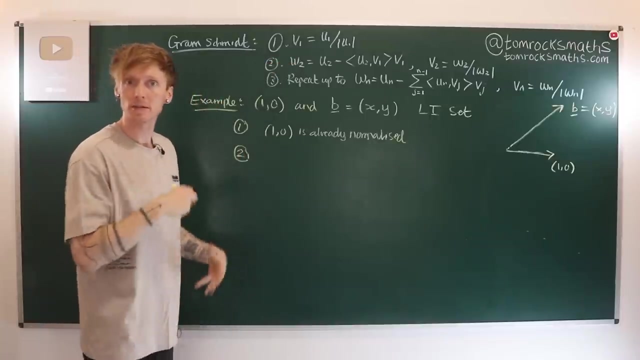 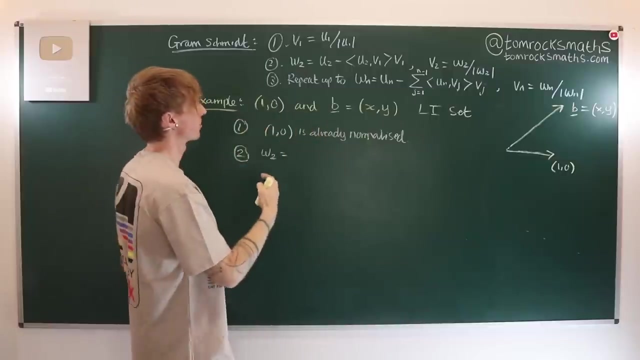 our vector b, which is going to be at the location in the 2D plane. Okay, now for step two. we need to compute this intermediate, So let's start with that. So w2, the intermediate is given according to the Gram-Schmidt procedure. Follow the algorithm, It's u2, which is b. 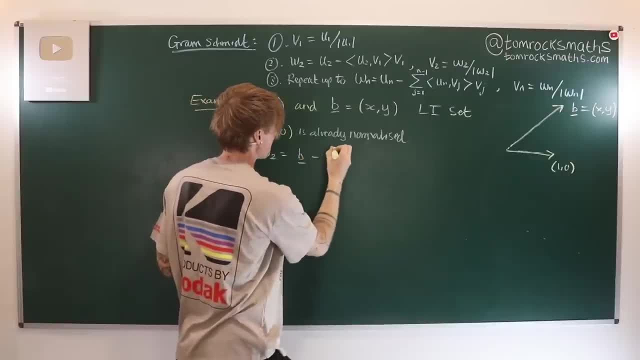 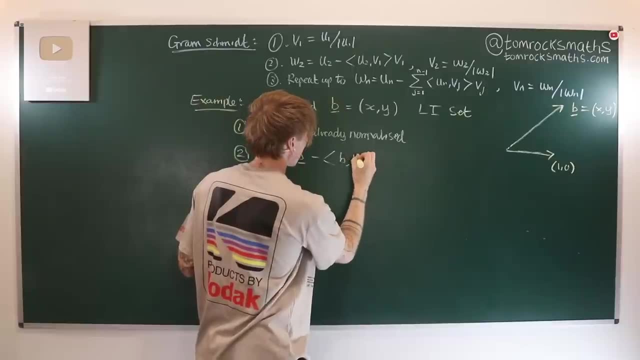 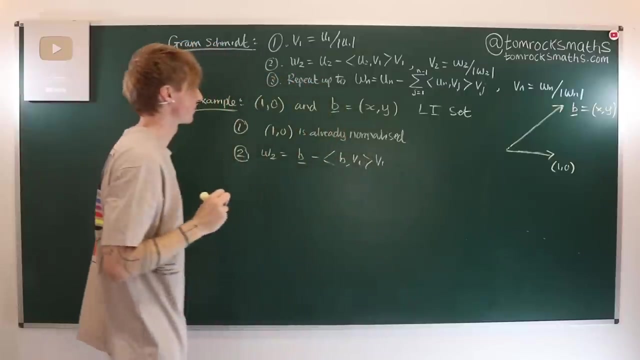 so it's our vector b minus the inner product of b, along with our first vector, which is- I will just call it v1 for now, but we will substitute in in just a moment and then we multiply by v1.. So this is now going to look like the vector b. well, that's x, y. 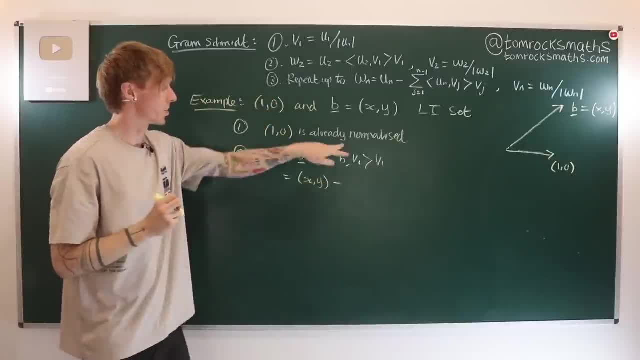 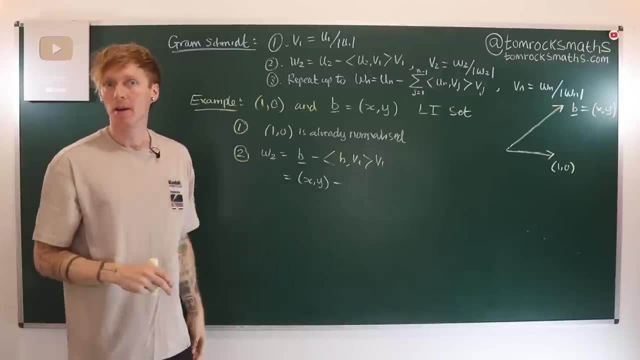 then we subtract off the inner product of two vectors. Now we're in the 2D plane, so the inner product here is the dot product- would be the standard one to take. So let's take the dot product. So this is now b dotted with v1, so that means we do. 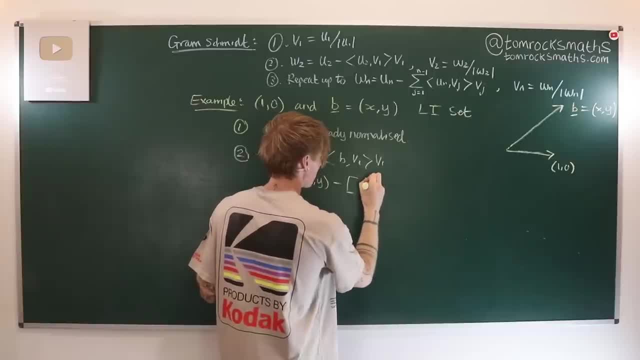 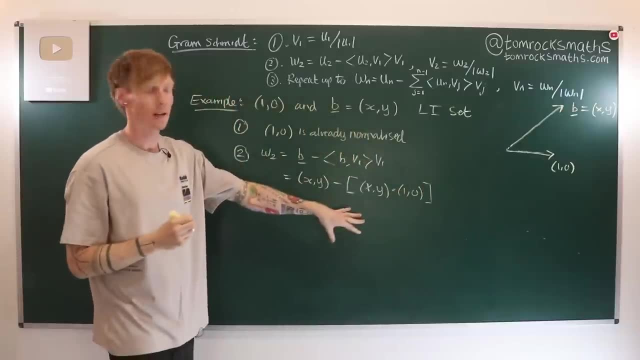 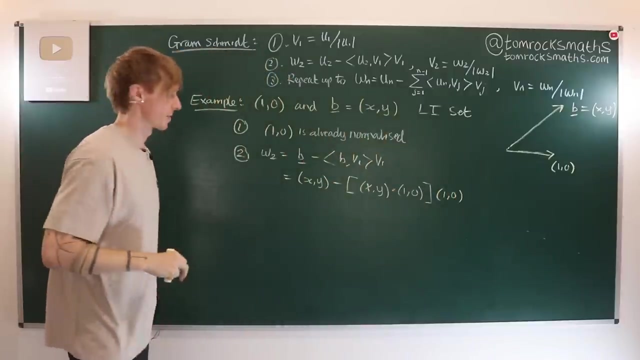 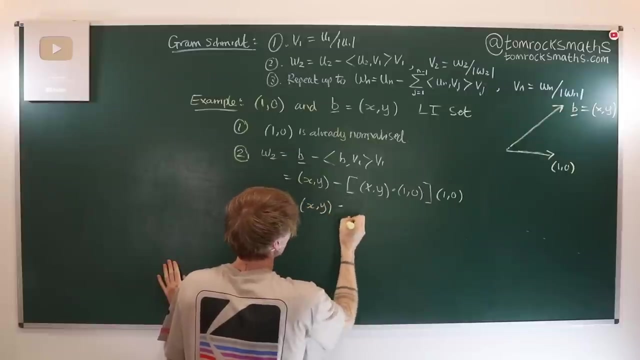 I'll put this in square brackets: b, which is given by x, y dotted with one zero, and then that gives us a scalar which then multiplies the vector one zero. So again, computing this explicitly, we can say: well, that is now equal to x, y minus. so we've got x, y dotted with one zero. 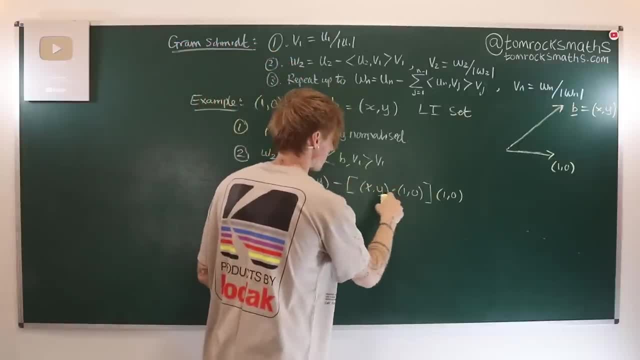 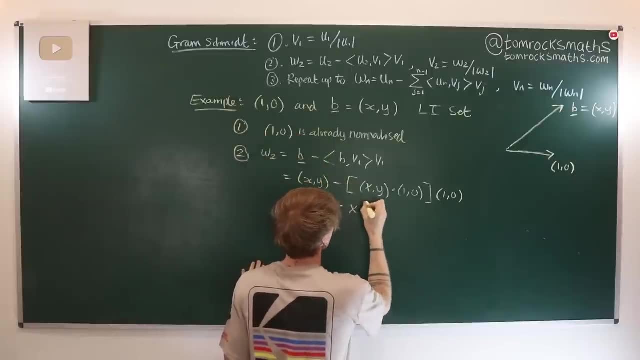 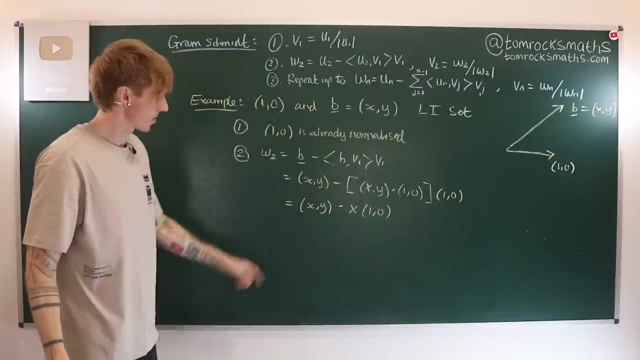 but one zero. that just gives us x times one plus y times zero. so that's just giving us x. So that's giving us minus x multiplied by one zero. So this bit in here just equals x. so now I've got x y minus a 0. 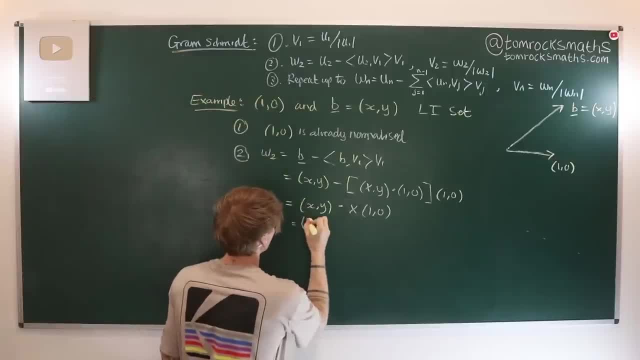 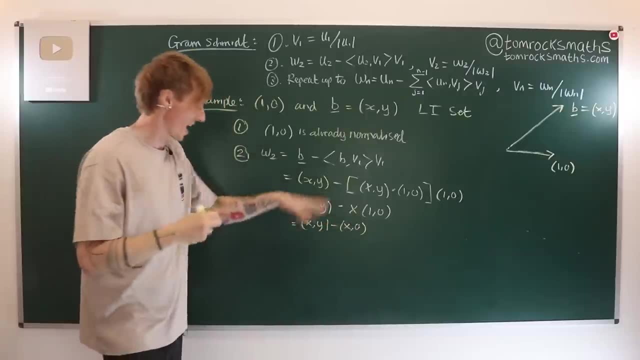 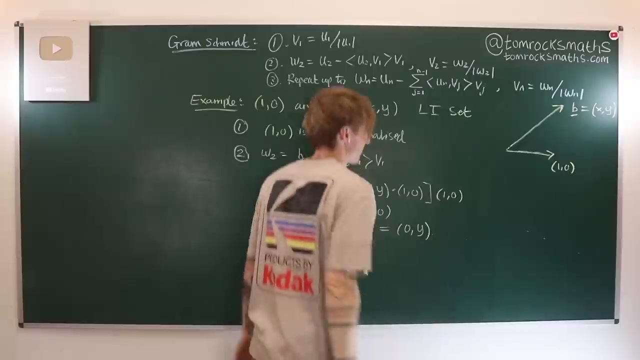 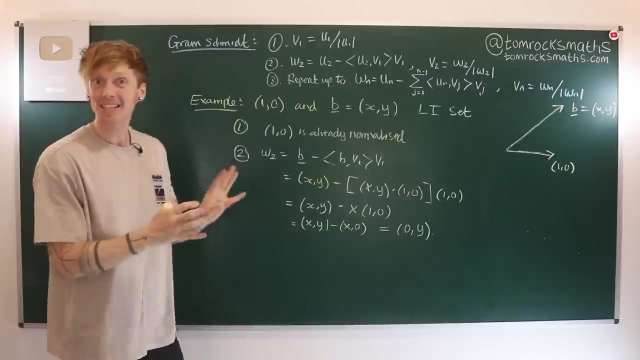 x times that. well, that's just. that's just the same as x y minus x zero. and so we can see now that we lose the x, So the x bit disappears and what we're just left with then is going to be zero comma y. So what we've done through this projection and subtraction aspect of the Gram-Schmidt- 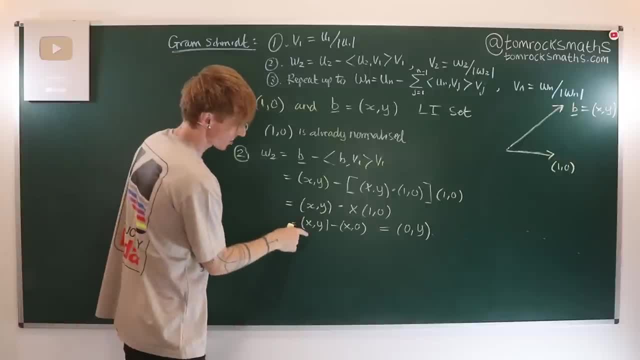 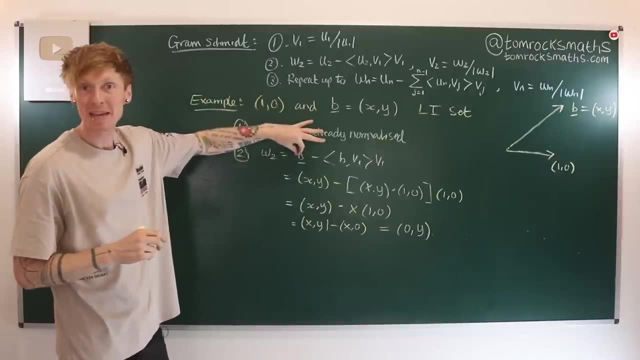 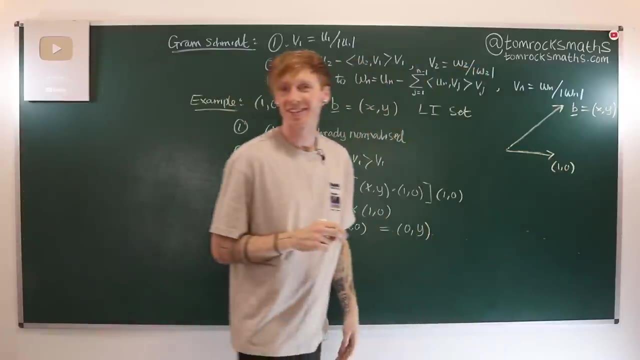 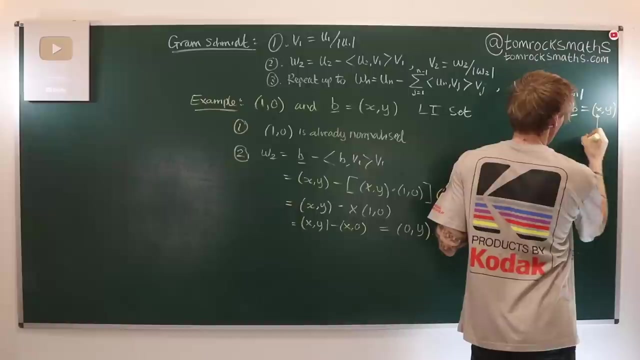 procedure. what we've done here is actually subtract away the x component of our general vector b. We've removed all of the component of that that was in the other vector, v1.. So b itself has two components, where the first one, this is the amount of v1.. Now this is, of course quite specific. 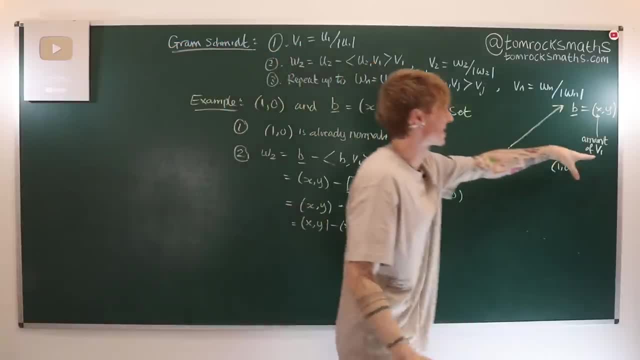 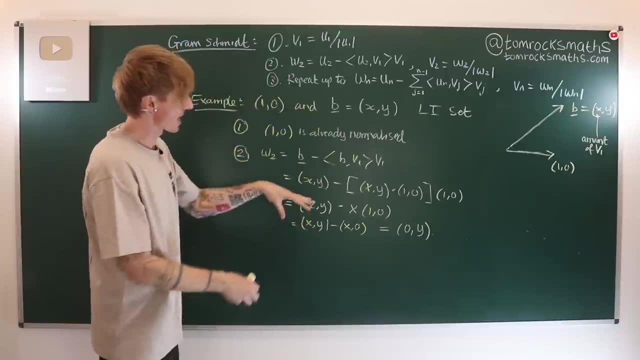 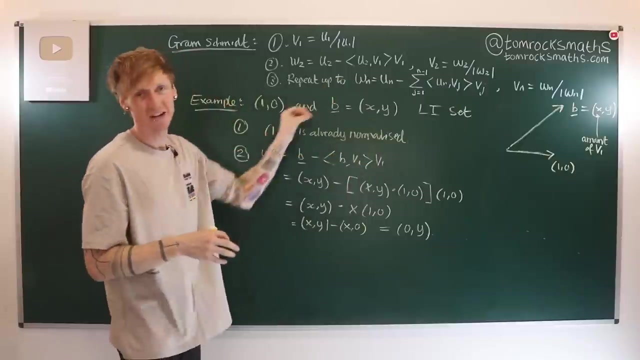 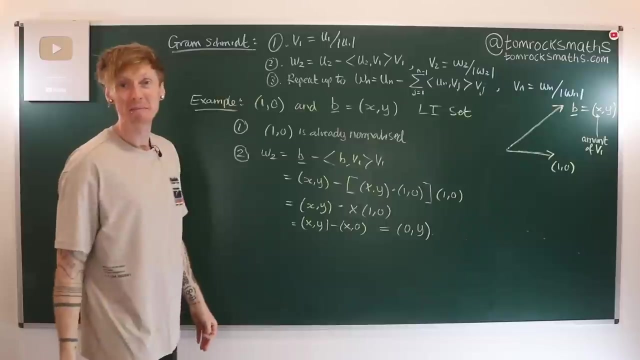 to this example, where v1 happens to be exactly the x-axis, but this works more generally. So what we're doing again is we're subtracting off the amount of b that's in the direction of our other vector so that we can make them orthogonal. We're removing that component. 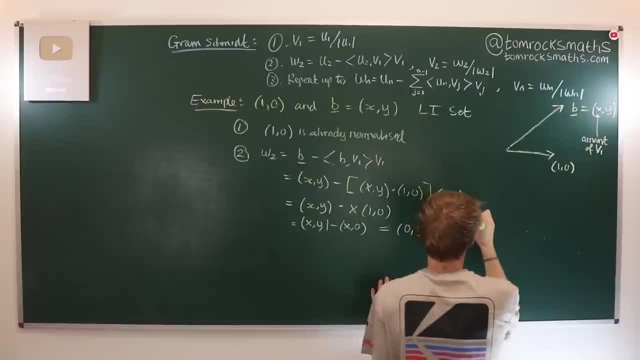 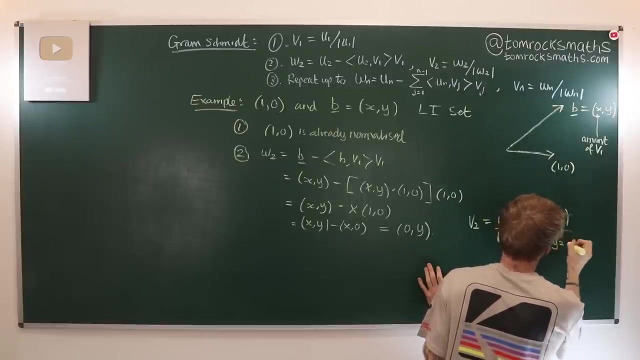 because now of course this is w2, so we can say: well, v2 then is just w2, divided by its norm, but w2 is zero y, so the norm of that is actually just going to be square root of y, squared, which of course is y, so we just end up with zero one to be our other. 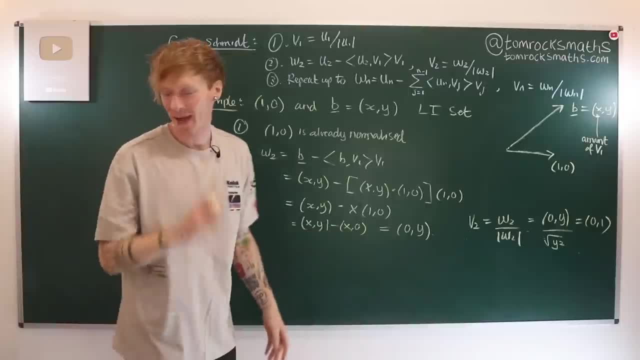 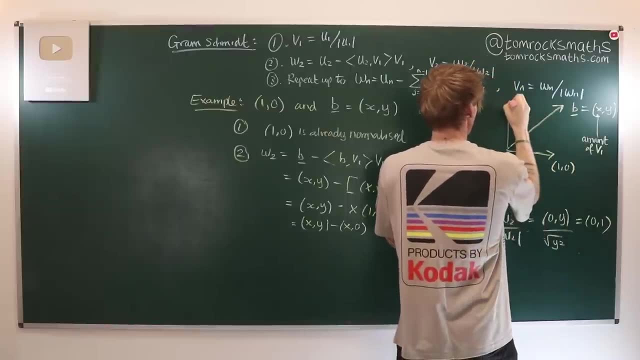 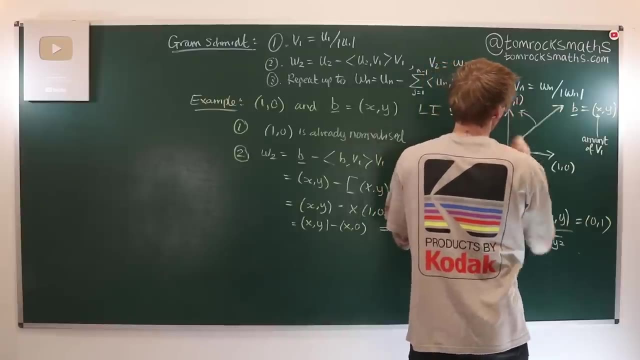 orthonormal vector, which, of course, is exactly what we expected. So what we've done is actually move, or rotate b to actually move, like so it's moved that way, and now we end up with the zero one. And now we've got our two vectors that are at right angles to one another. they are orthogonal. 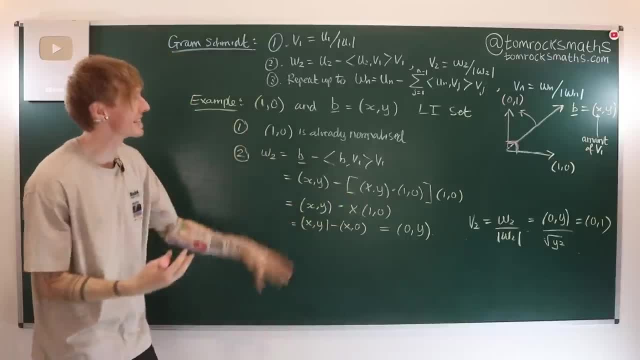 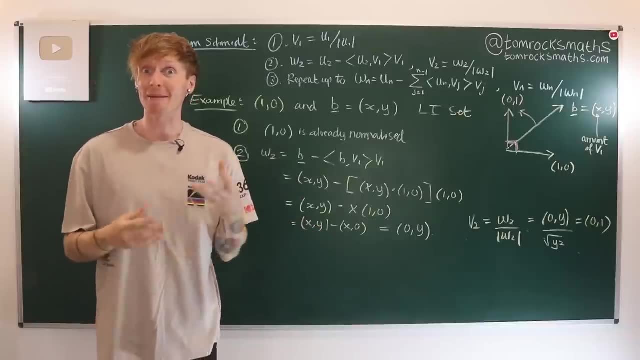 and they both have length one, which are the two properties we need for it to now give us an orthonormal basis. So that's Gram-Schmidt. We started with a pair of linearly independent vectors. We apply steps one and steps two of the algorithm, as there are only two vectors- to orthonormal. 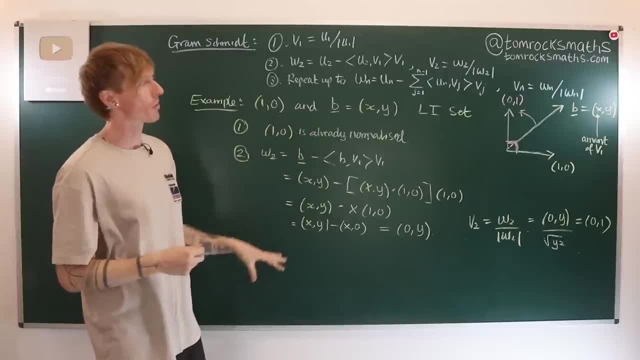 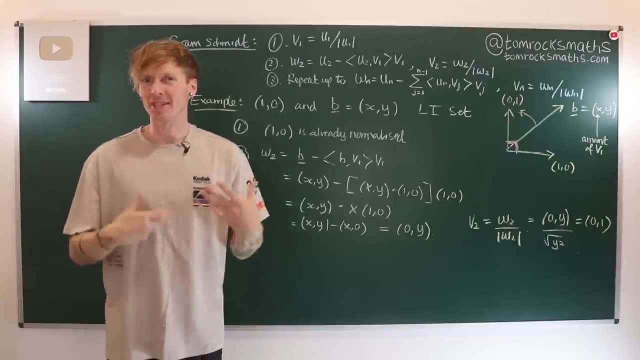 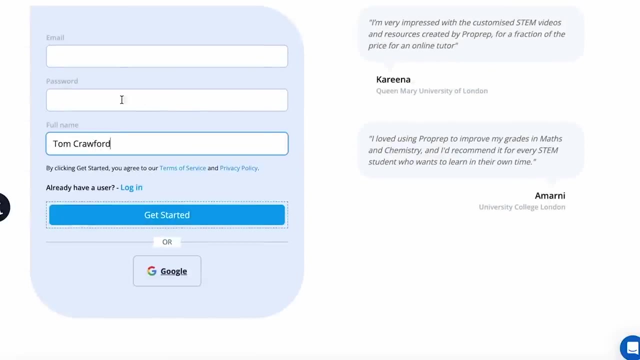 orthonormalize and we end up with our orthonormal set: one zero and zero one. As usual with the Oxford Linear Algebra series, there is another video explanation available to all of you via ProPrep, which you can access for free by signing up for a 30-day free trial using the link in the video description. 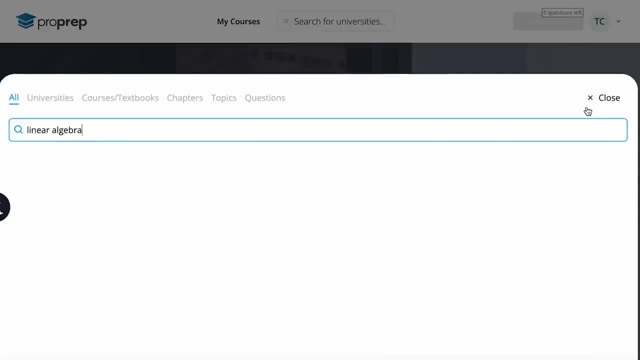 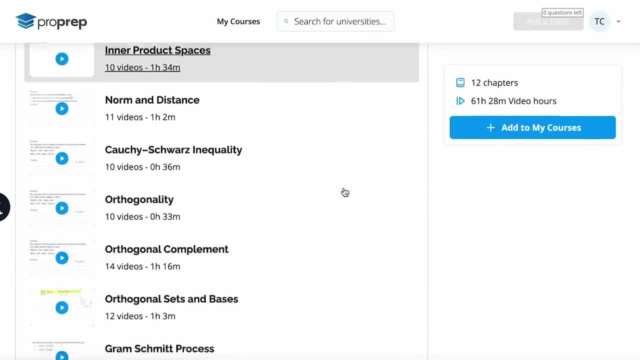 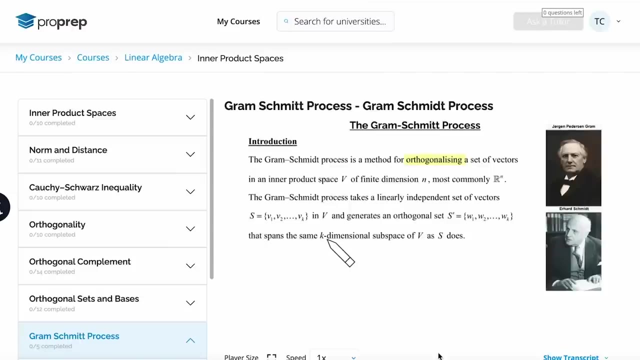 ProPrep is an online resource which provides video tutorials for students looking to improve their skills in stem-based subjects. Alongside an alternative explanation of the steps in the Gram-Schmidt process, there are four exercises, each with full video solutions. The first two extend the example we've just looked at of the Cartesian plane. 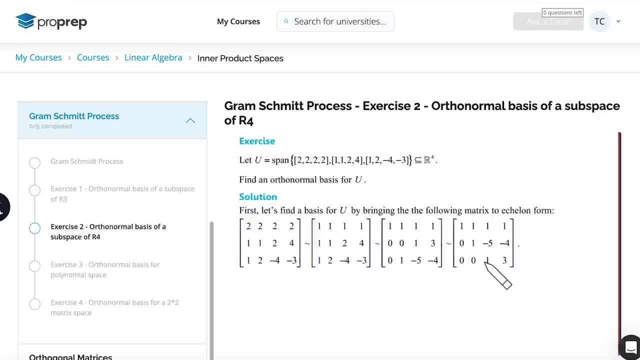 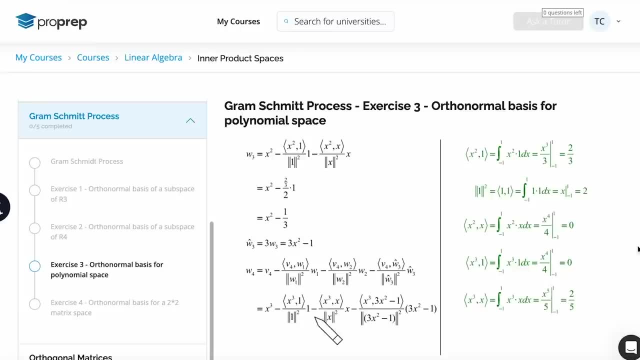 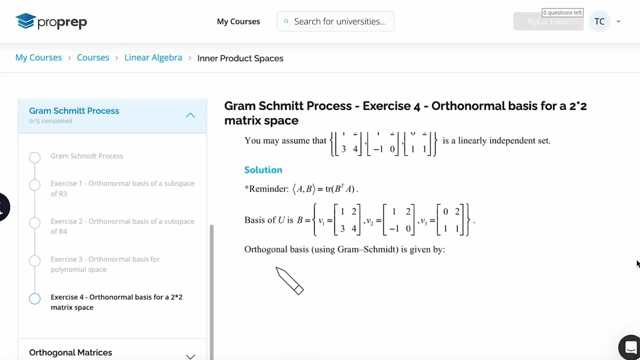 to three and four dimensions. Next, we have an interesting example on the polynomial inner product space, where the inner product is defined via an integral. And finally, we have an example involving matrices with another type of inner product, this time defined using the trace of a matrix product. 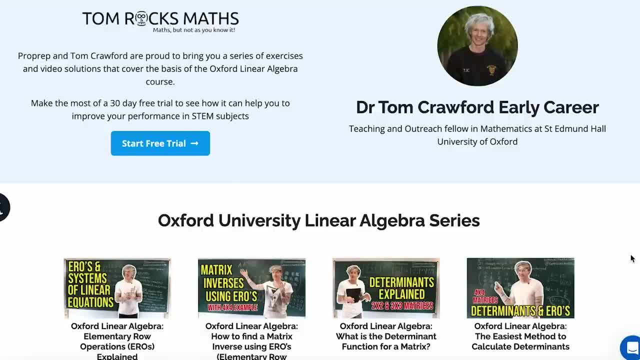 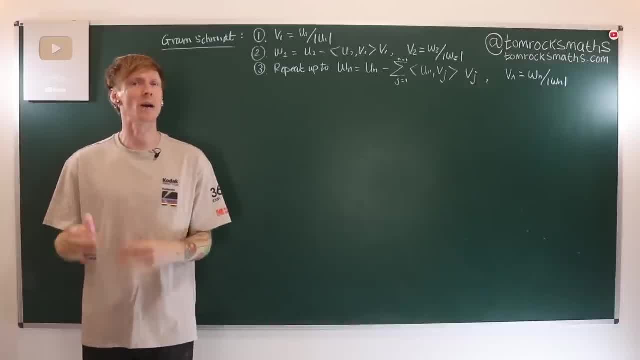 Just click the link in the video description to get started with your 30-day free trial right away. Now that we've outlined the procedure and hopefully have a better feel for how and why it works, let's work through a final explicit example. We've already looked at plenty of RN examples, both here and in the 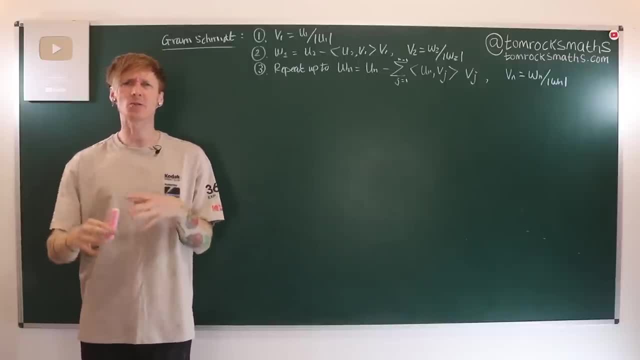 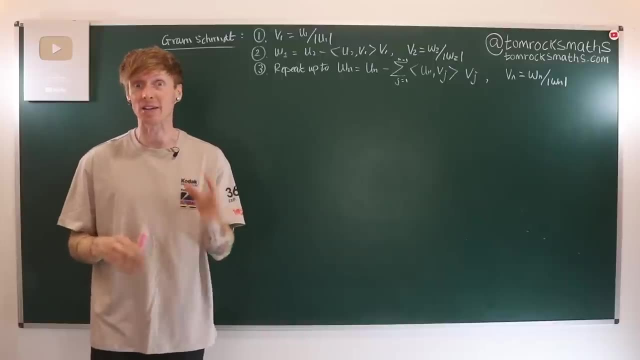 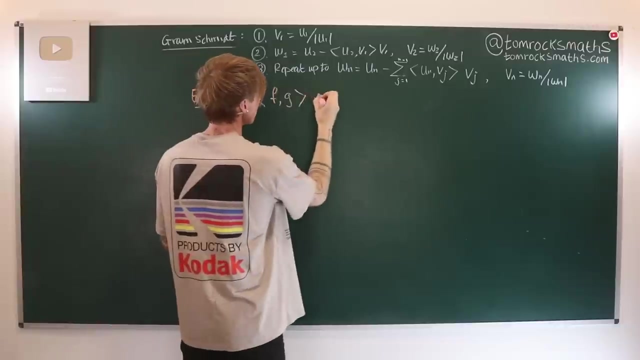 previous video In the previous video on inner product spaces. so let's do one in the polynomial inner product space instead, where the inner product here is going to be defined as follows: So if I have my two polynomials, f and g, then we say the inner product of them is going to be given by. 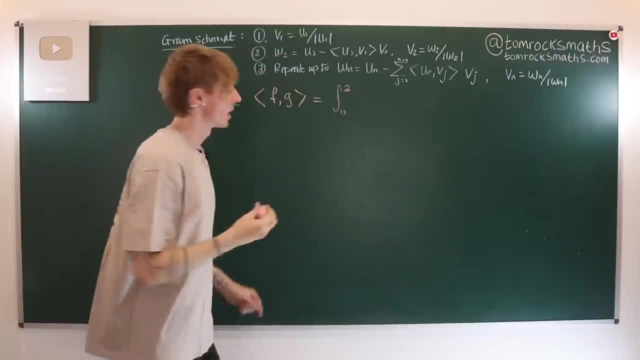 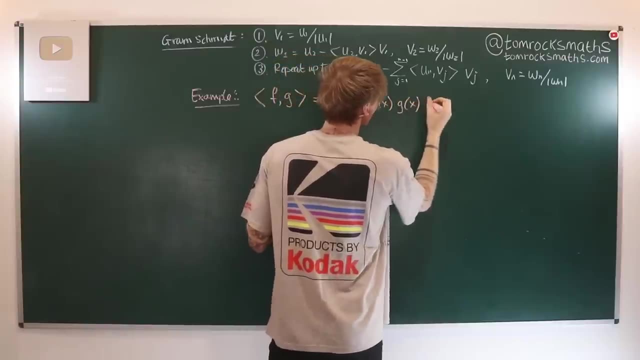 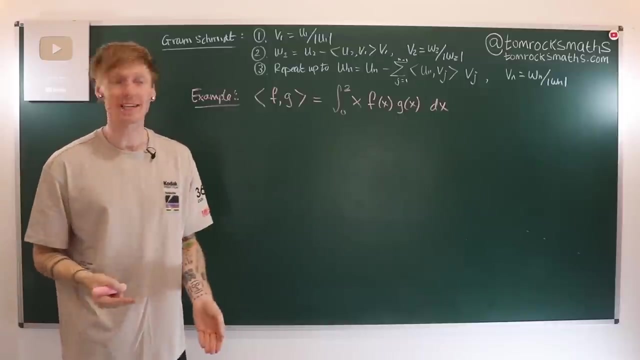 the integral from 0 to 2. then we have a weight function x, f of x and g of x. Of course we integrate with respect to x. So this is slightly different to any of the previous examples we've seen, because now we have this weight function x inside the integral. 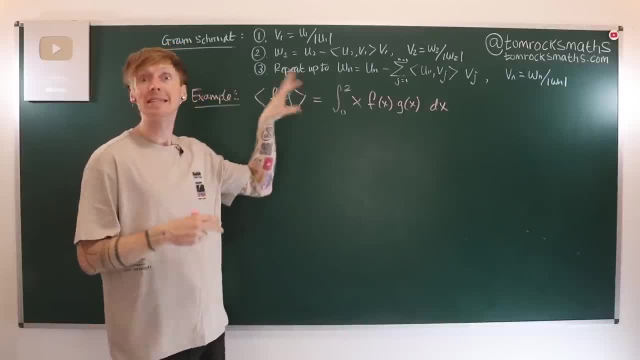 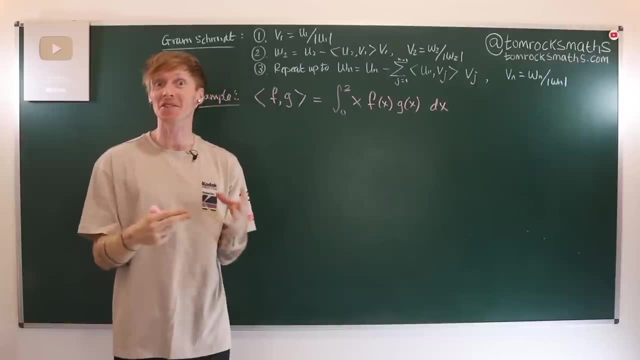 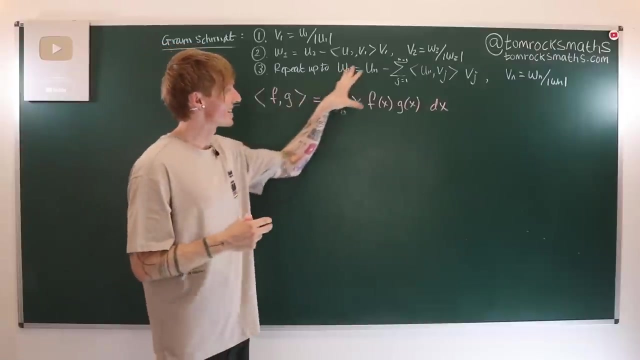 Now I'm not going to go through the details to show that this does indeed define an inner product, but it is a highly recommended exercise for the viewer, particularly for those of you who are still getting to grips with what we covered in the previous video on inner product spaces. So you want to check that this is indeed. 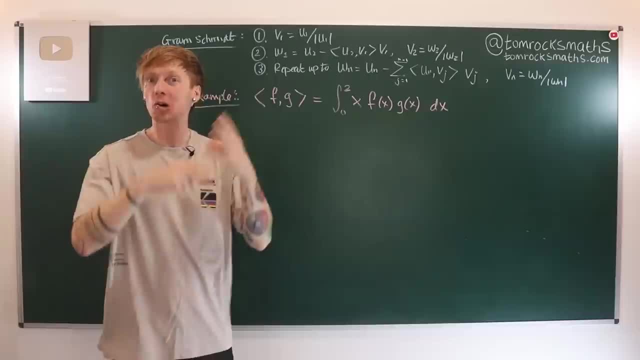 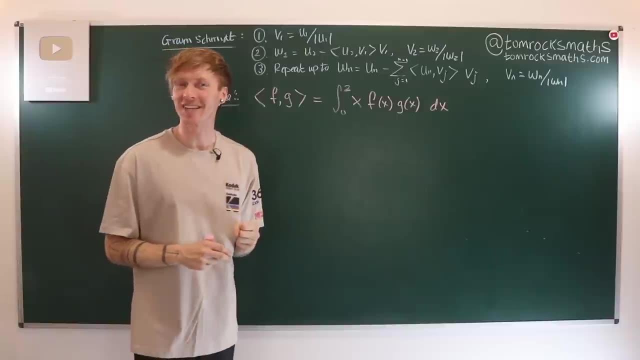 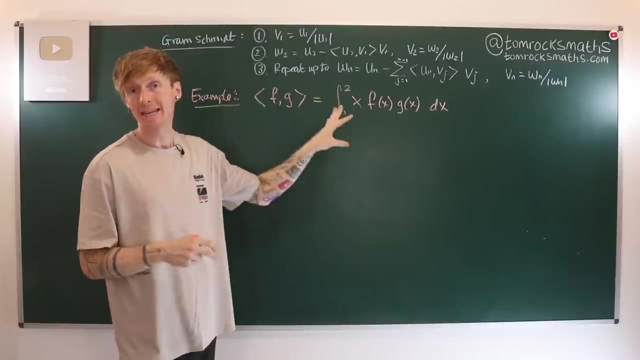 linear, it's symmetric and positive definite according to the inner product definitions from last time. But what we are going to do here, because it's the focus of the video, is actually to construct an orthonormal set for this inner product space. So we're going to start with a linearly independent set. 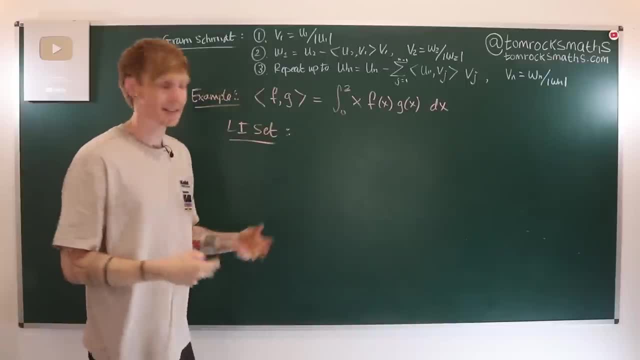 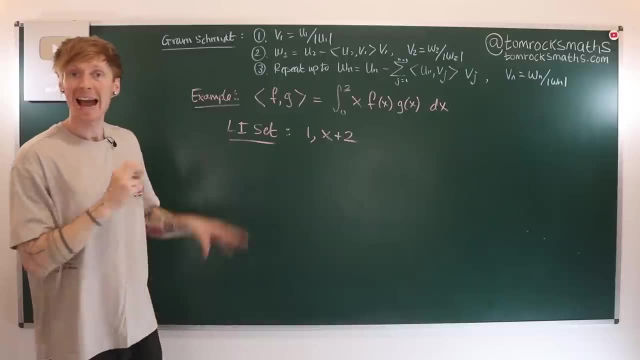 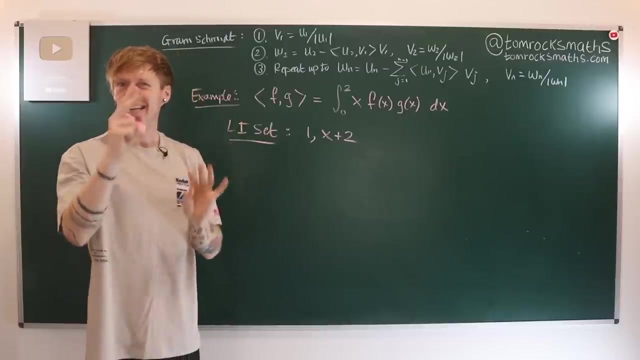 and I'm going to suppose that my linearly independent set is going to be 1 and 2. And x plus 2.. Again, I'm not going to check that this does indeed define a linearly independent set. Again, you can check this for yourselves. 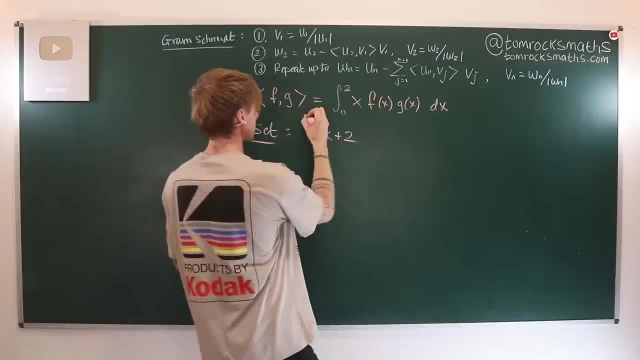 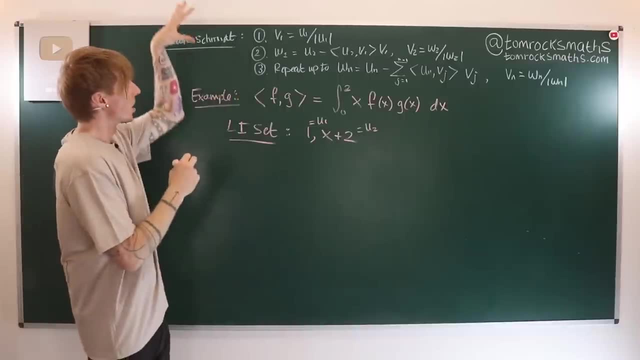 What we want to do is take these two vectors, so let's call this one u1 and this one u2.. Take these two linearly independent vectors and we want to follow the Gram-Schmidt procedure and hopefully get something at the end which is going to be an. 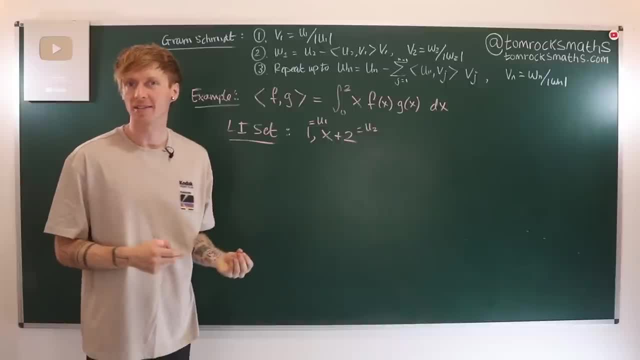 orthonormal set or an orthonormal pair of vectors. So step one is to normalize our first vector. Now you may look at this and be like, oh, it's already normalized, it has length one, but that would be using the traditional definition of length. 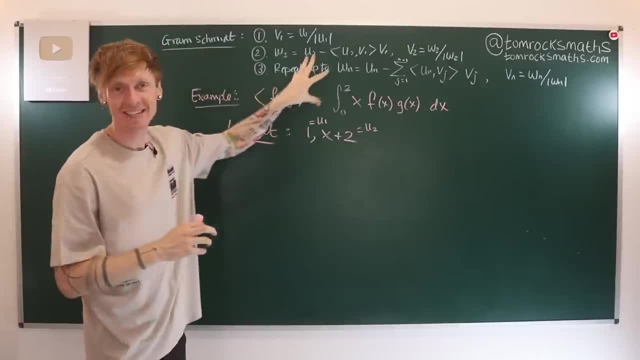 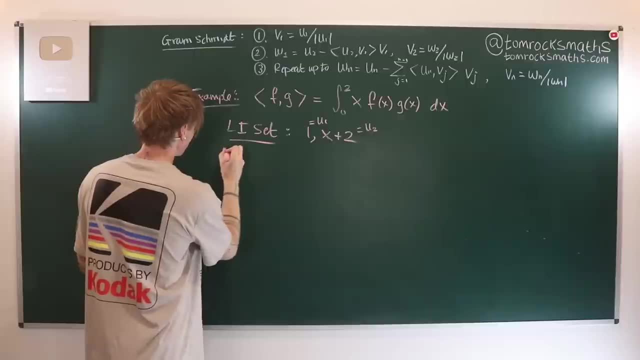 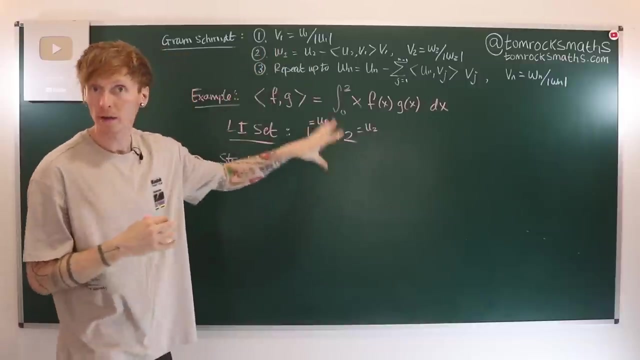 Here our length is defined by this inner product. so we have to check that is indeed the case. So step one: we want to compute the norm of one using this inner product and then of course divide by that to get a normalized vector. So we want: 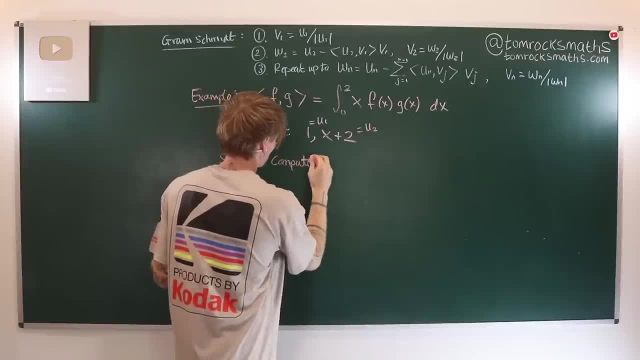 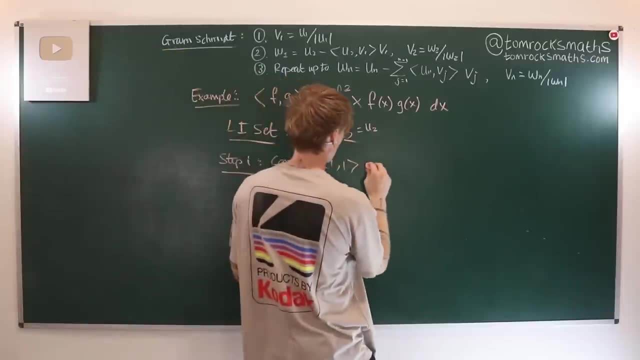 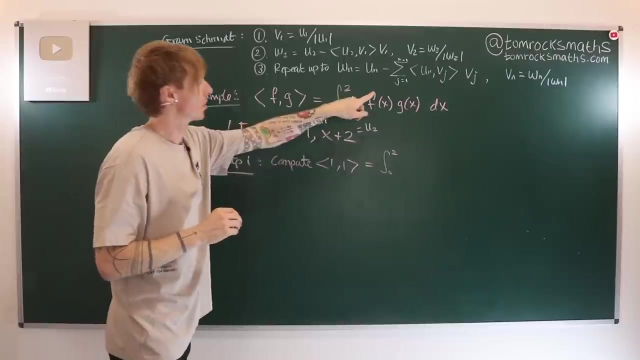 to compute the inner product, again using this definition, as written on the board here, of one and one. So what's that? That's the integral from naught to two of x, our weight function multiplied by one, multiplied by one, We're integrating x between zero and two, so that is x. 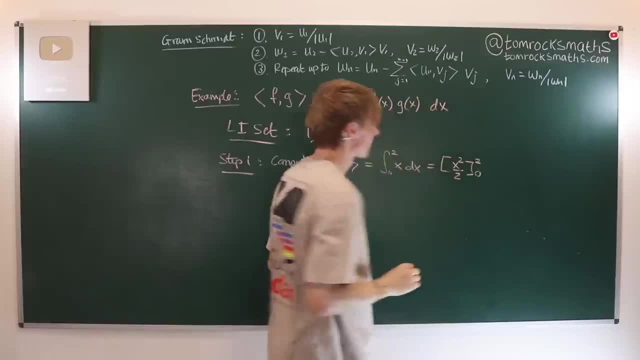 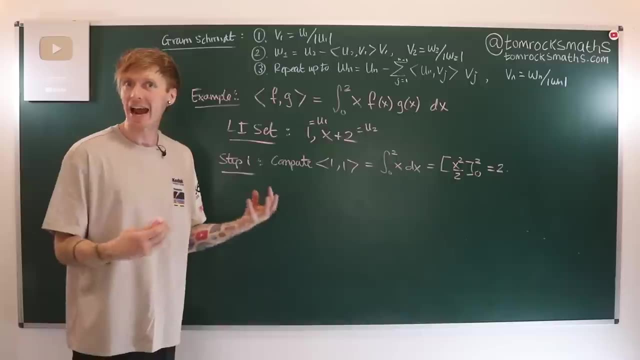 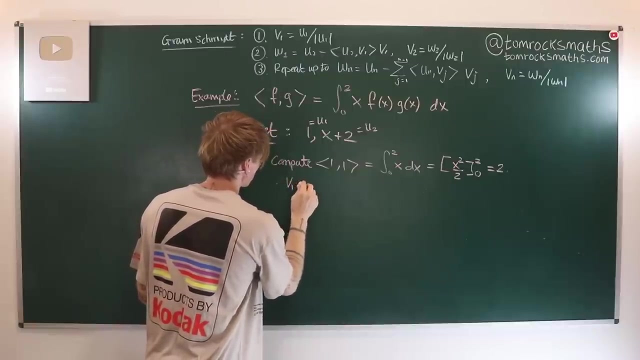 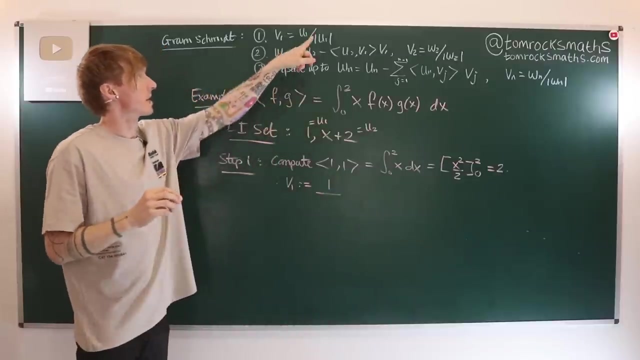 squared, divided by two, evaluated between two and zero. So we're just going to get two is going to be the answer. So, therefore, to normalize our first vector, we need to say so. therefore, v1 is actually going to be defined by the first vector, one divided by the modulus of one. So that's going to be one divided by the modulus of one. 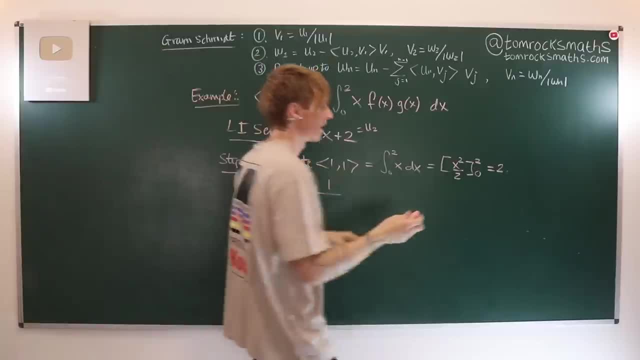 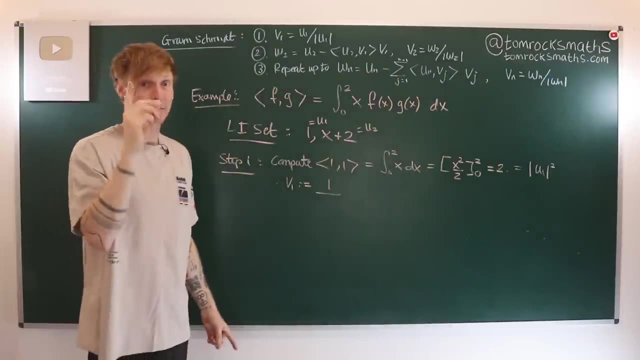 So that's going to be one divided by the modulus of that vector. Now what we've calculated here is actually the modulus of u1 squared. So we have to remember- and this is important, lots of my students miss this- you have to remember to square root this: 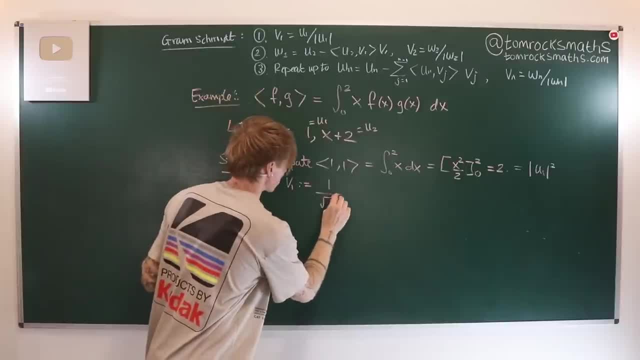 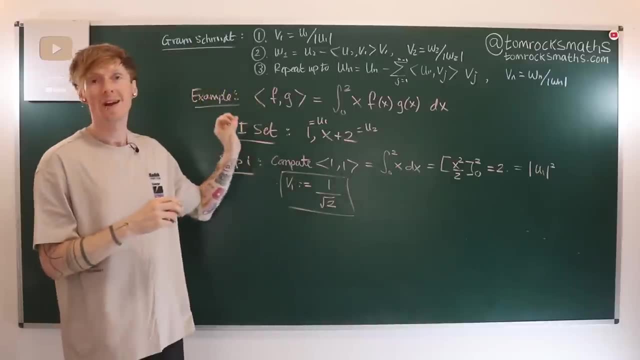 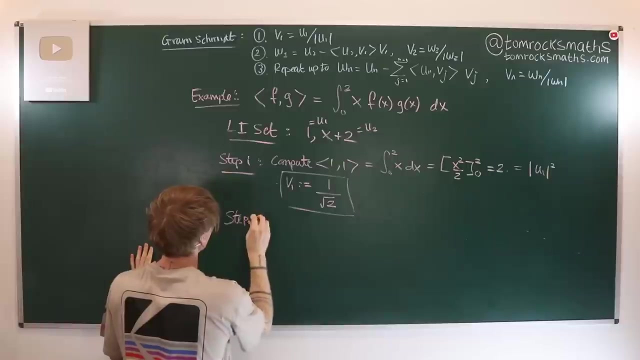 answer. So the modulus of u1 is going to be the square root of two. So this is in fact going to be our first orthonormal vector. We now continue with step two, which is to first define our intermediate. So step two. 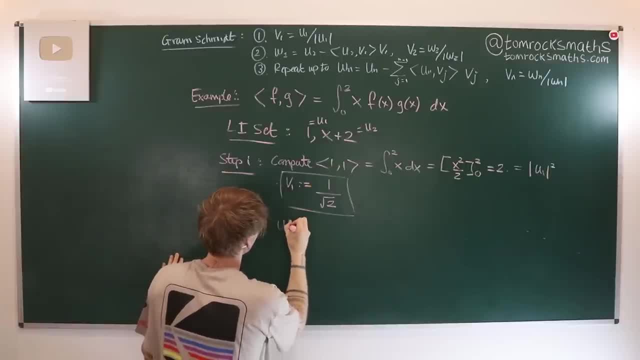 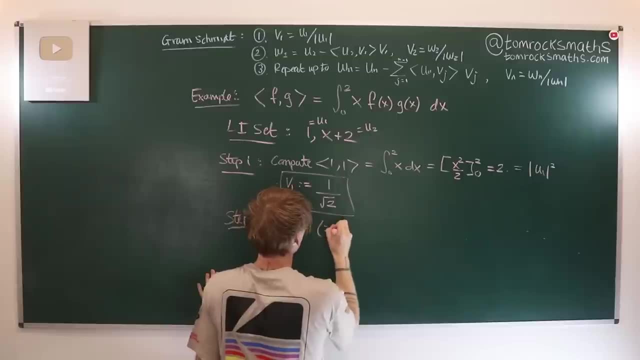 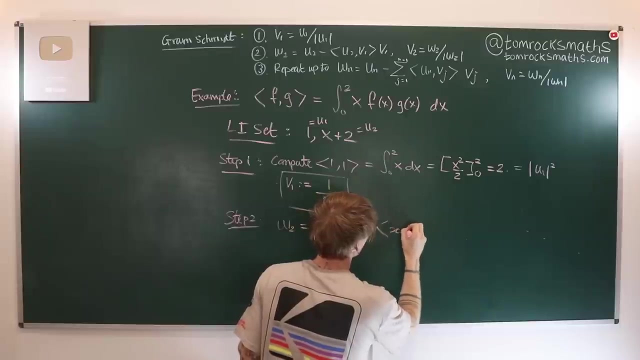 We are going to therefore consider our w2, which is going to be equal to u2, which is x plus two. So we have x plus two, and then we subtract off the inner product of x plus two with v1, which is one over root two. 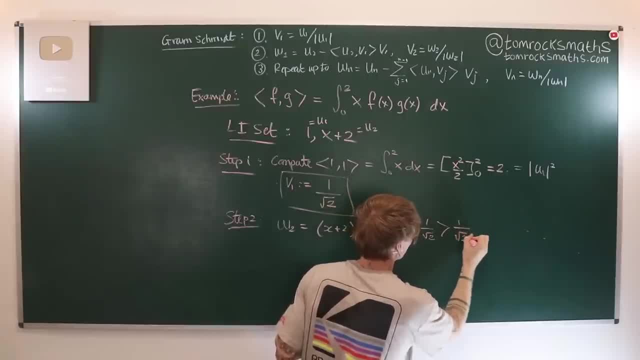 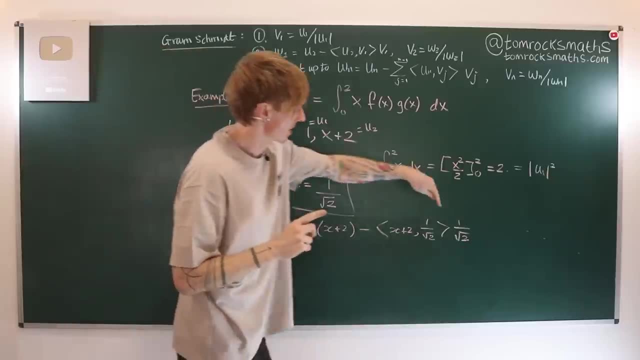 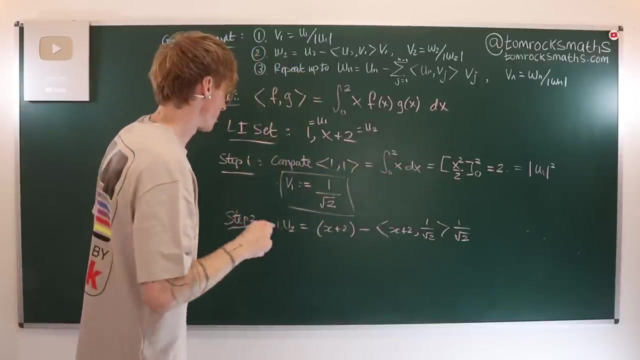 And then we multiply that whole thing by one over. So I'm going to simplify things a little bit here, just to help me out. If I take this one over root, two inside, that will just give me a one over two inner product. So this is going to now require me to calculate. So we compute. 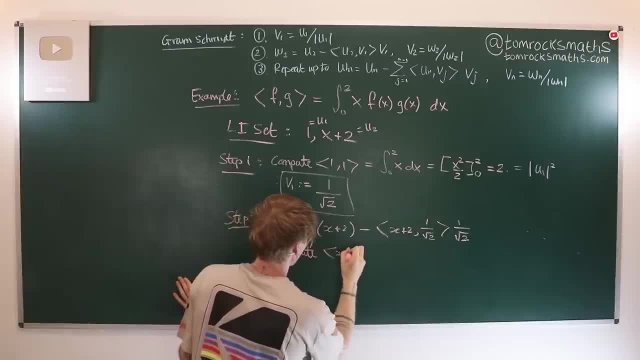 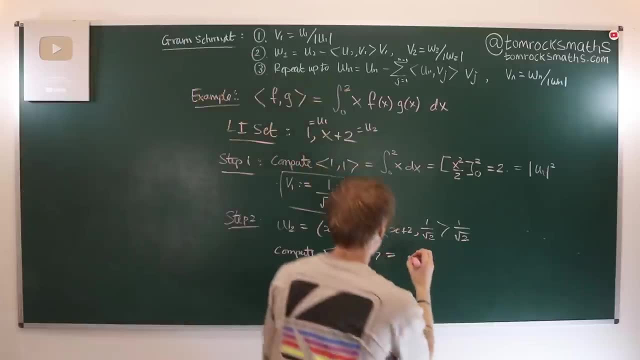 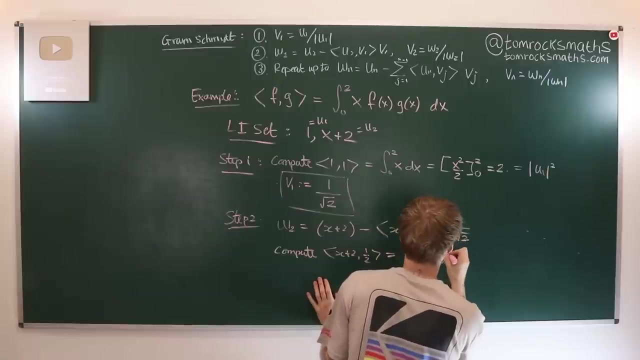 therefore the inner product of x plus two, along with a half. So again using our definition up here, that's going to be b. Pull the half out and we've got the integral from 0 to 2 of x times x plus 2.. So that's x squared plus 2x. 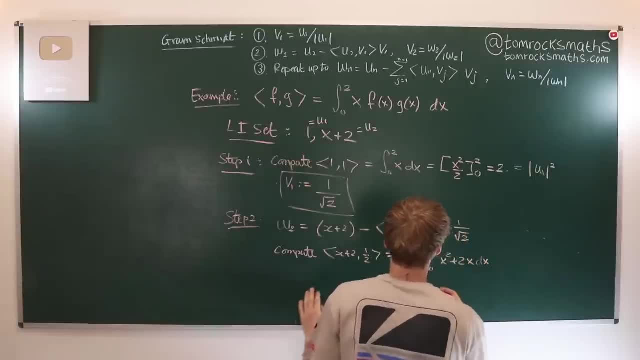 with respect to x. So we again leave the half outside. We do that integral and that's going to be x cubed divided by 3 plus x squared, And that's between 2 and 0.. So that's going to give me a half. 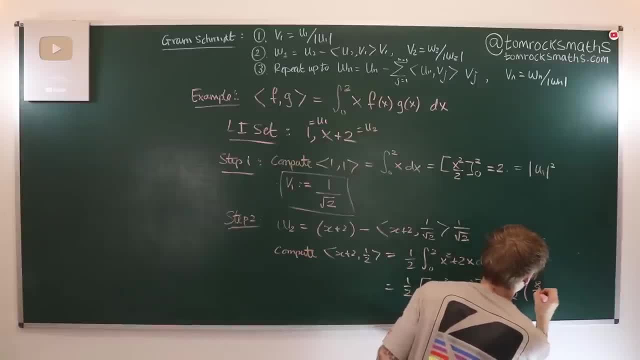 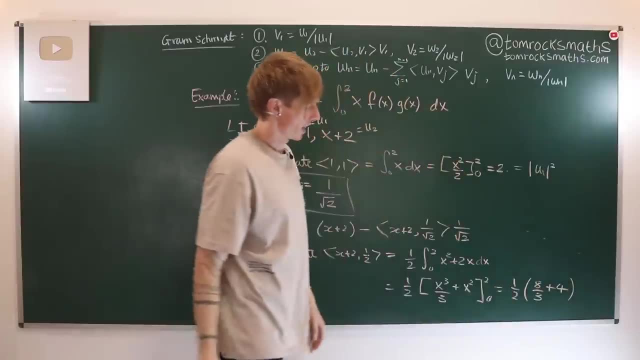 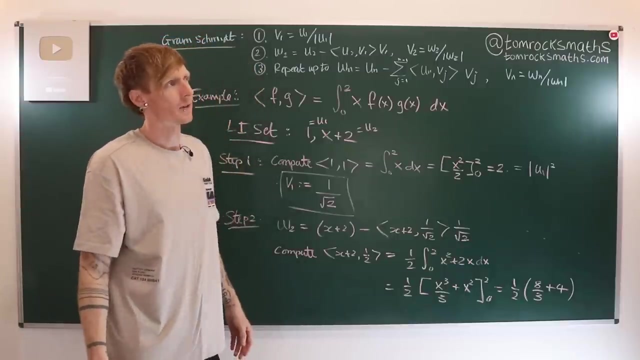 multiplied by eight thirds plus four. Okay, so that is the same as four thirds plus two, which is 10 over 3.. Do I agree with that? Four thirds plus two is indeed 10 over 3.. Yes, so that's 10 over 3.. 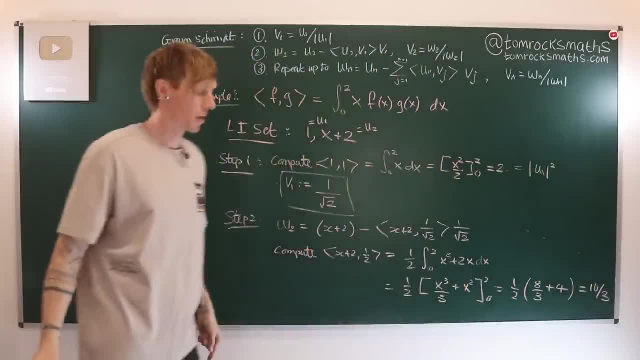 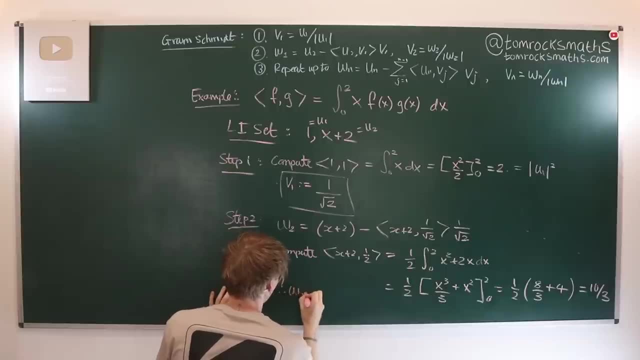 Okay, so we now go back and plugging this up here. So therefore, w2 is x plus two minus the thing I just computed, So minus 10 over 3.. So that whole thing, then, is actually just going to now give me x plus two minus four thirds. 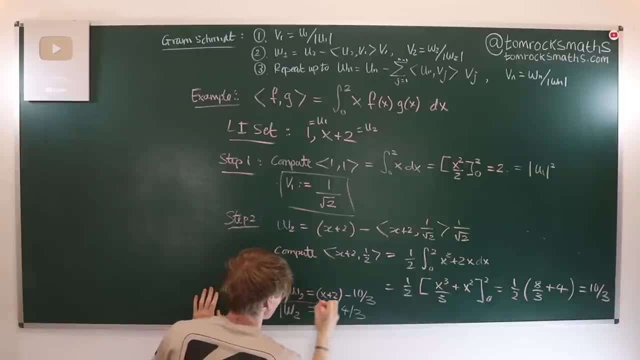 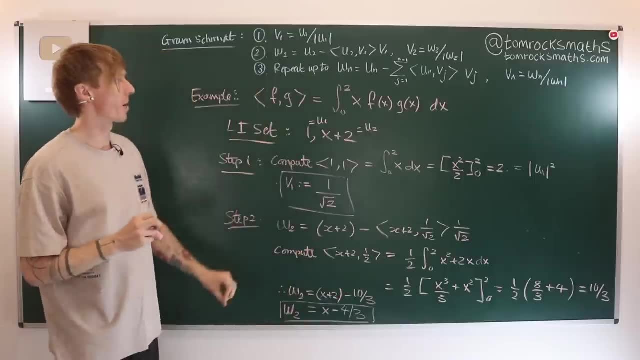 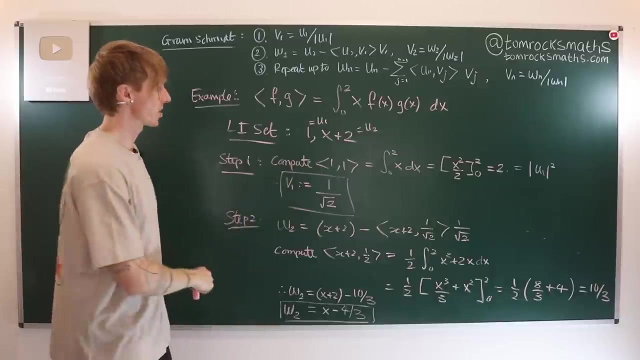 So that one is w2 here, which is not yet the answer. of course, This will be orthogonal to our other vector 1 over root 2, but is not yet normalized. So we have w2.. We need to normalize it. So, carrying on over here, 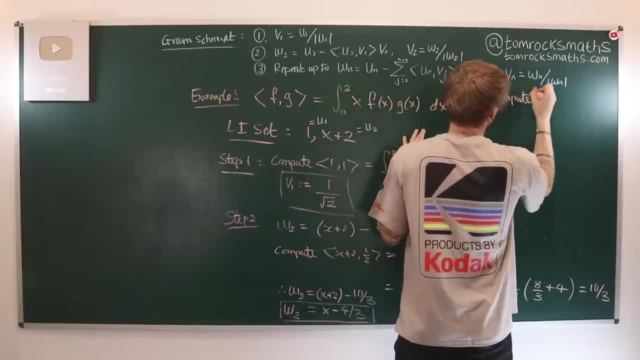 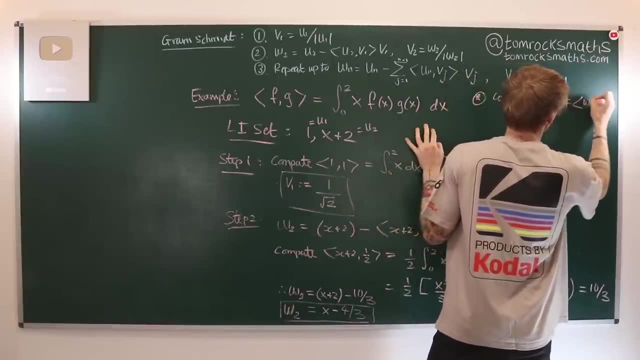 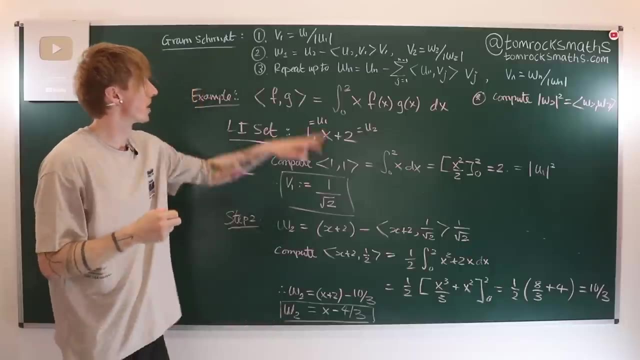 we need to compute w2 with itself. So the modulus of w2 squared is the inner product of w2- w2.. So again, according to our definition, we've got x minus four thirds with itself and with this x. So we actually want the integral. 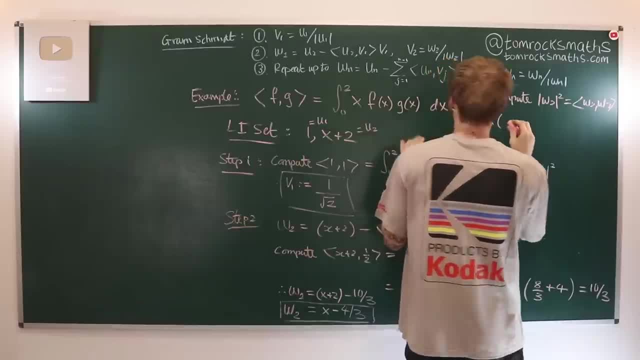 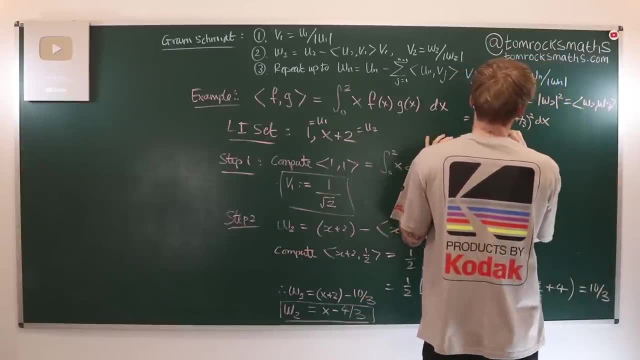 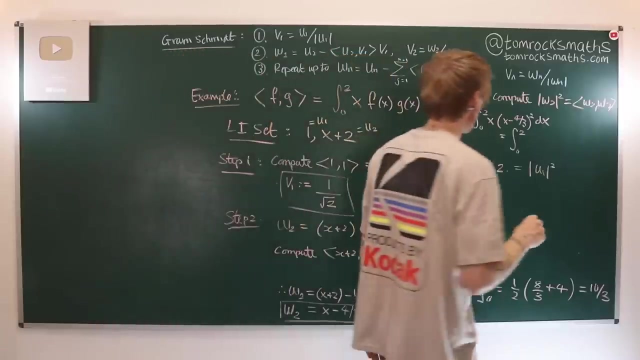 from 0 to 2 of x times x minus four thirds squared. Okay, dx, so that's going to be the integral from 0 to 2.. I'm going to do the square inside the bracket, so that's going to give me a an x squared. 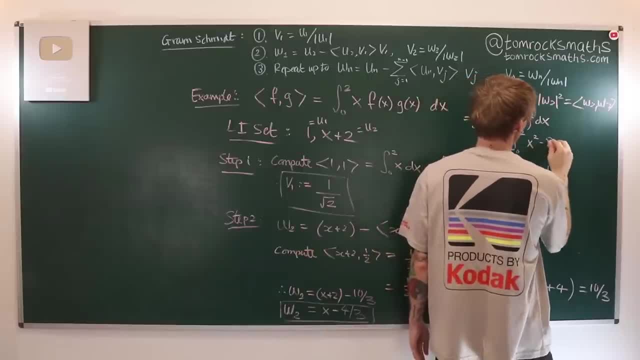 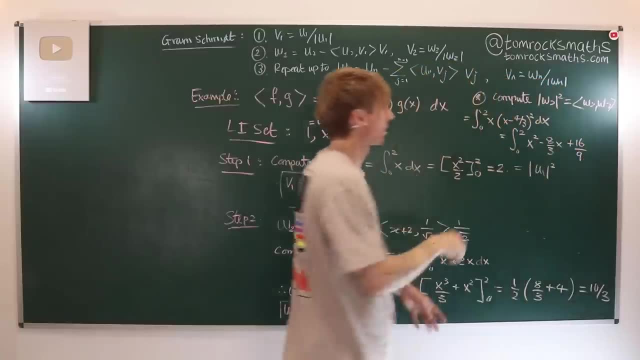 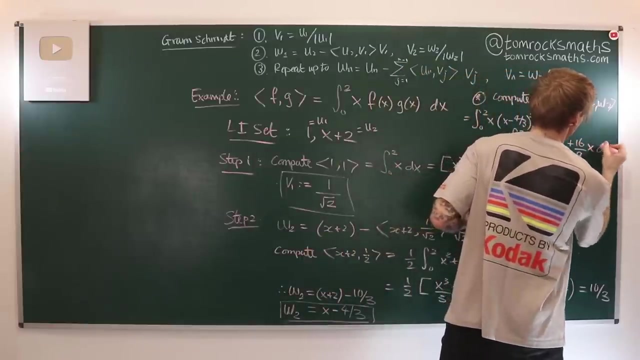 Minus four thirds x, minus another, so minus eight thirds x, And then it's going to be plus 16 over 9. And then all of that square bracket is multiplied by x. So that's actually an x cubed, That's an x squared and that's an x dx. 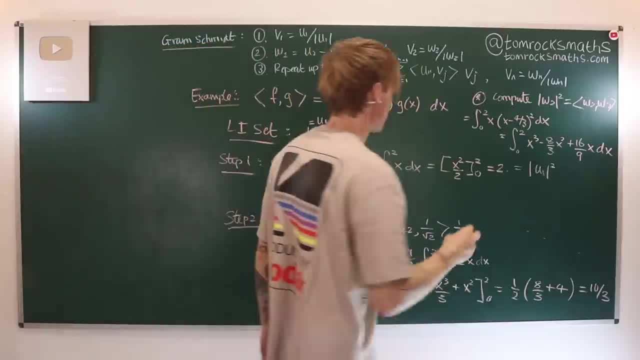 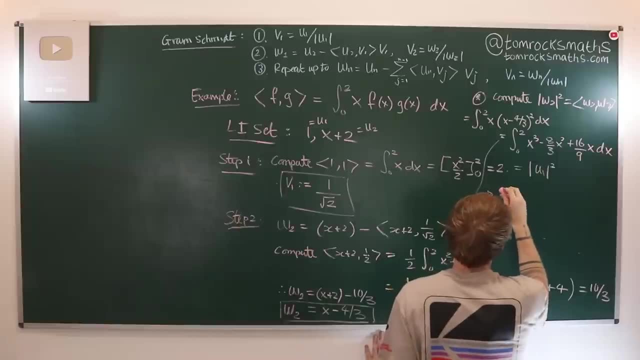 Now we can do the integral. So again, if I just kind of pull a little arrow down here, The board's getting quite crowded. So this is now the integral. It's now going to be equal to What have we got? We've got x to the 4 divided by 4 minus 8 over 9. 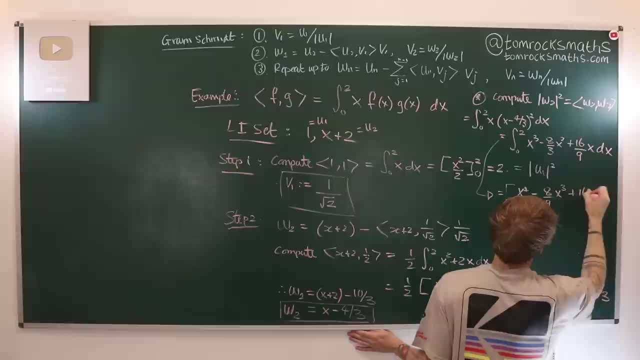 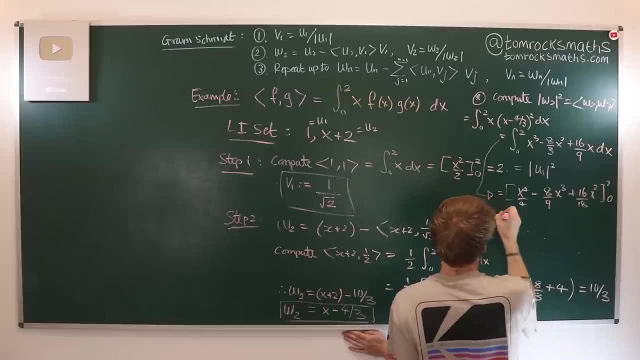 x cubed plus 16 over 18, x squared between 2 and 0.. So putting all of that in, that's 2 to the 4 is 16.. So 16 over 4 is 4.. Minus 8 9ths, so minus 64 over 9.. 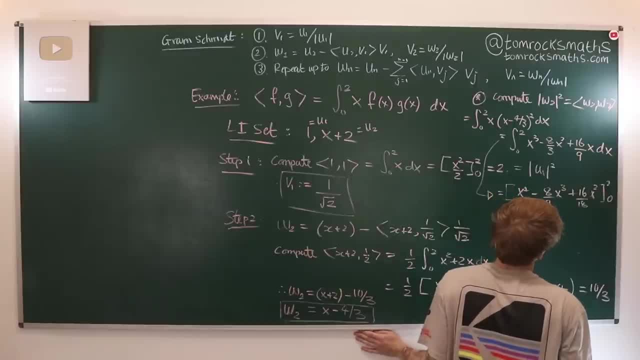 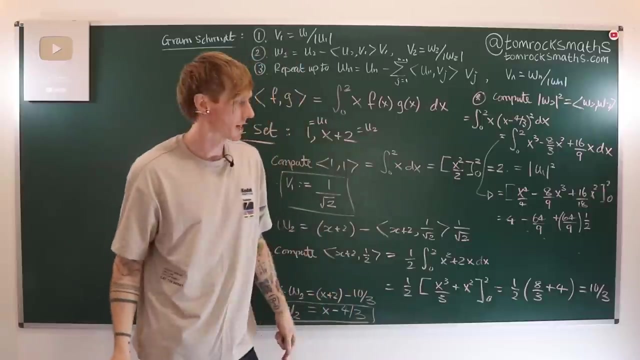 And then plus 16 times 4 is 64. So plus 64 over 18. So that's 64 over 9 times a half is what that is. So it's 4 minus 1, lot of 64 over 9 plus a half of them. 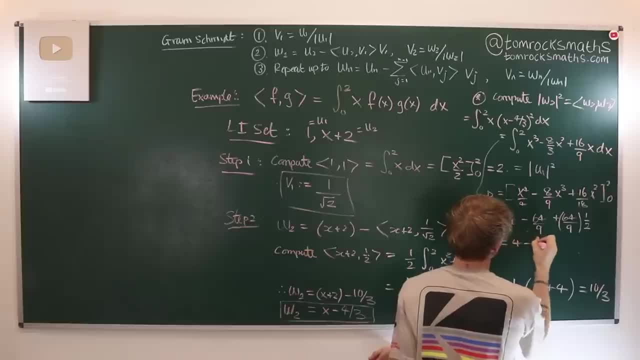 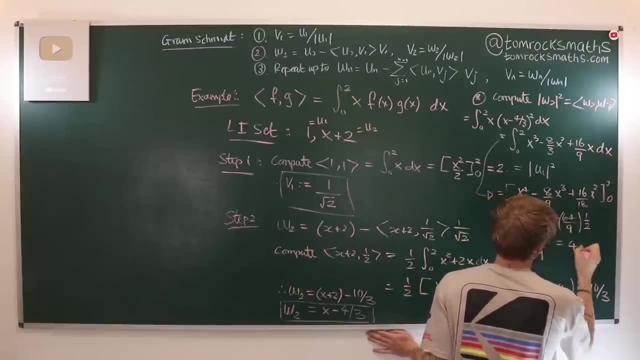 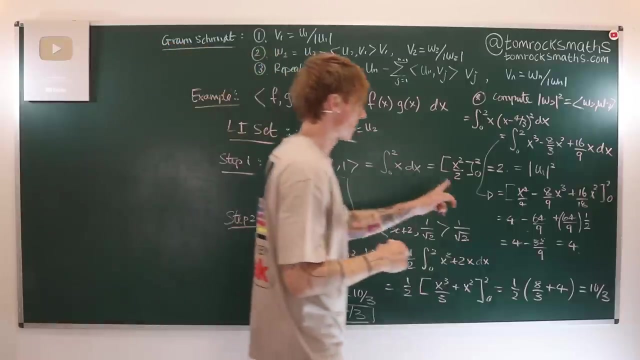 So it's 4 minus a half of that. so it's equal to 4 minus 32 over 9, but that of course simplifies to be 4. 32 over 9 is: oh, wow, and wait, they'll make that 36, that's four nines. 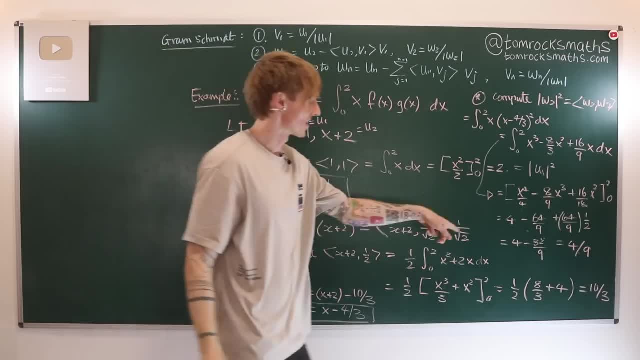 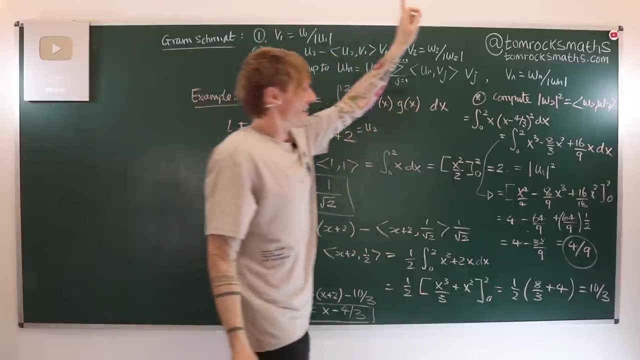 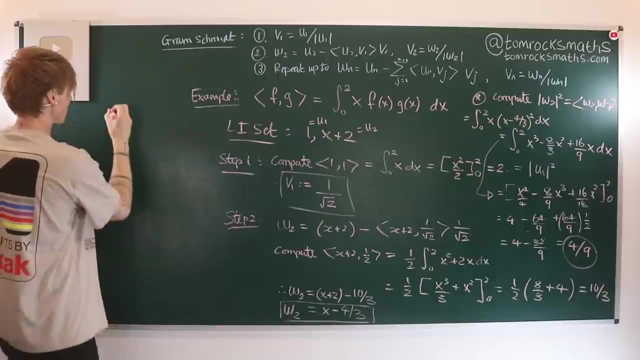 the four is 36 over nine. that's what i've done in my head. so it's 36 over nine minus 32, so it's four ninths. all right, so the value of mod w2 squared is four ninths. so we have to divide by the square root of that. so again, i'm going to squeeze it over here. 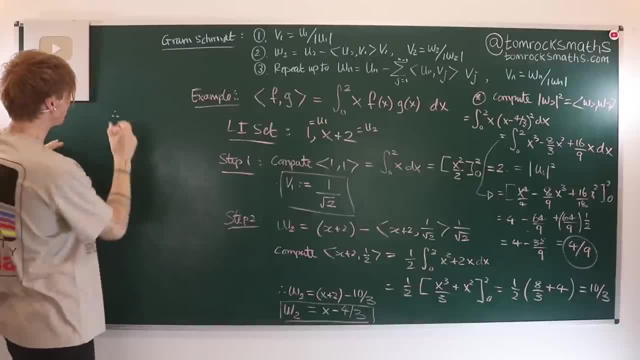 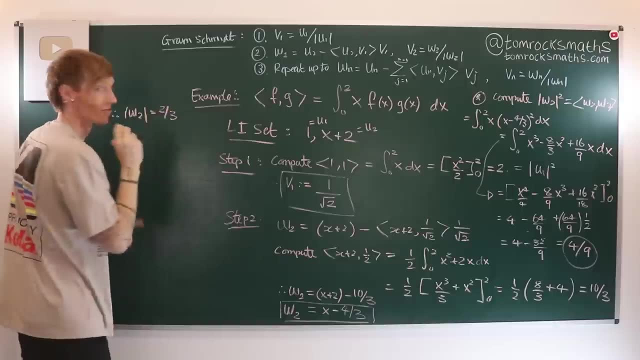 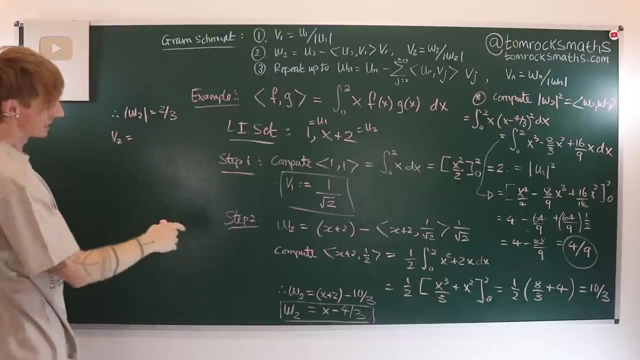 final step. a lot of work in this one, therefore, the modulus of w2 is the square root of that. so that's two thirds, which works out really nicely, and so therefore, finally, we can say v2. our final vector here is going to be x minus four thirds, and we want to. 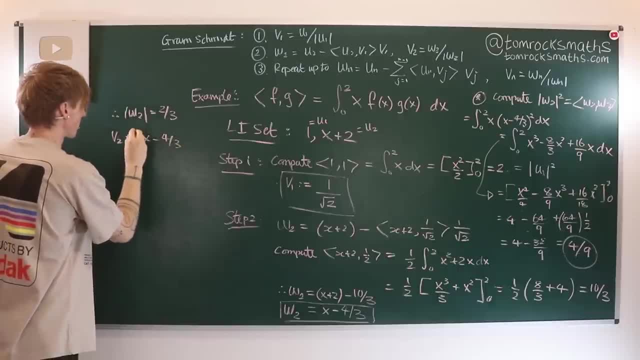 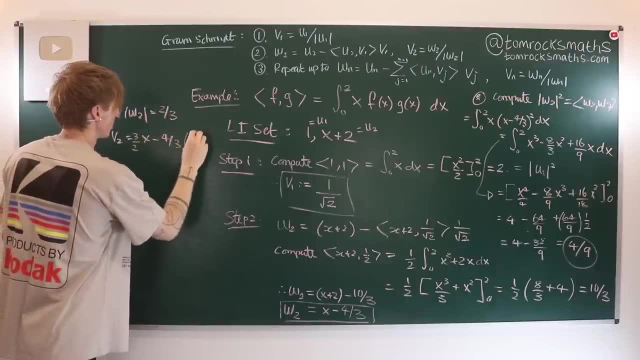 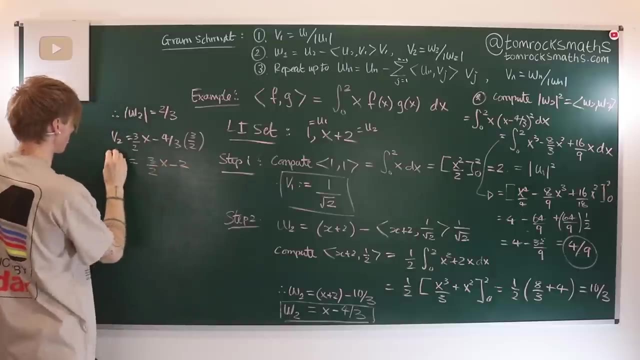 divide the whole thing by two thirds. so multiply the whole thing by three over two. uh, so three over two gives me four thirds times three over two. so that's going to give me three over two x minus two. i believe is going to be my final answer. 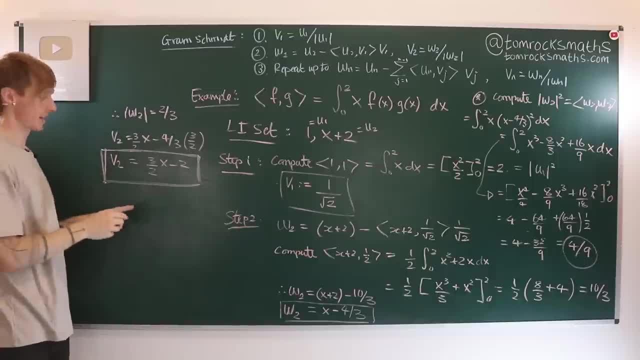 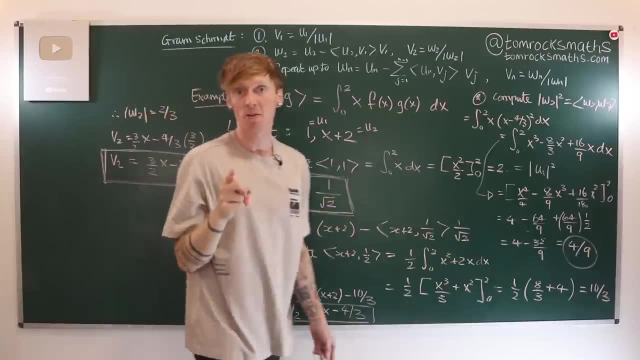 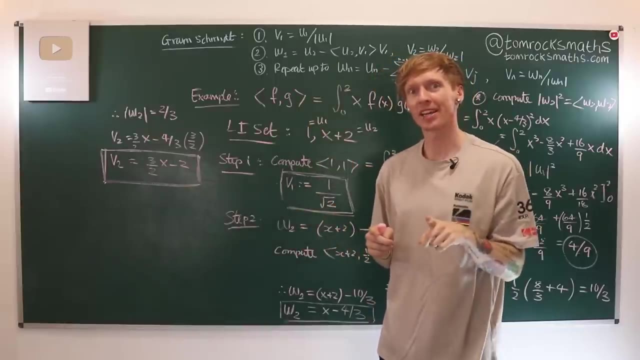 so i think i think my second orthonormal vector is three over two x minus two. my first one is one over root, two over here and, of course, as you might have guessed, i'm going to set this as an exercise for all of you watching to check my working. 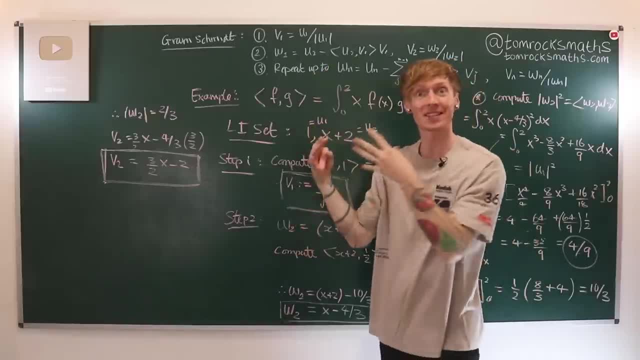 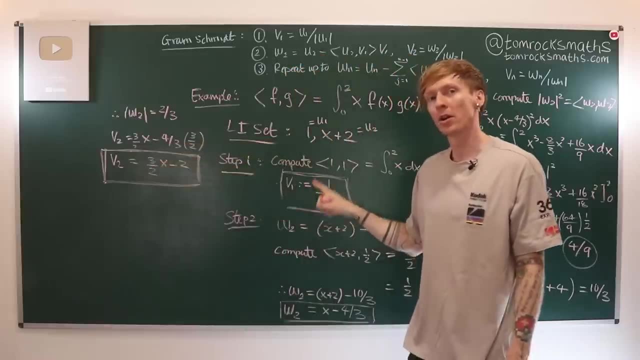 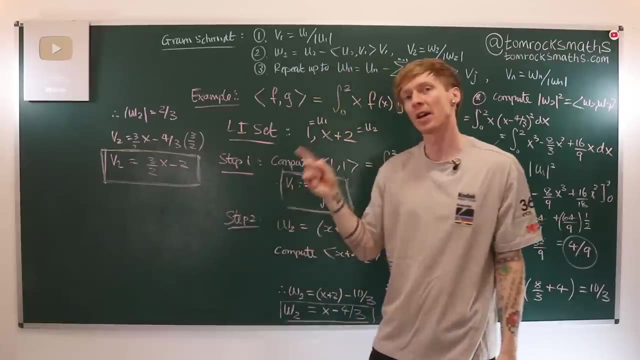 so, if i have done this correctly- and i have certainly followed the steps of graham schmidt, but if my algebra is correct- v2 in a product- v1- should give you zero, v1 in a product with its itself should give you one, and v2 in a product with itself should give you one.